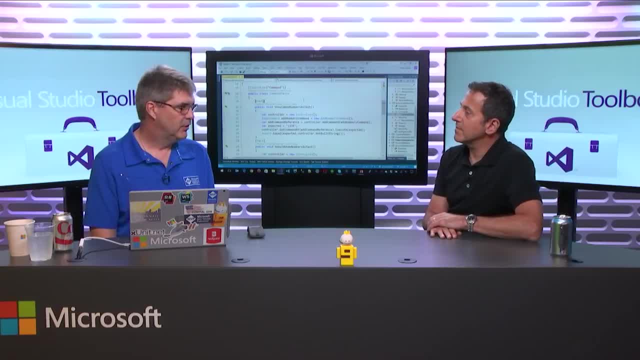 there might be screen doors, there might be pocket doors, but they're doors. The pattern that that's filling is providing an egress between two spaces that can be closed. So that would be the kind of the quote unquote design pattern concept. 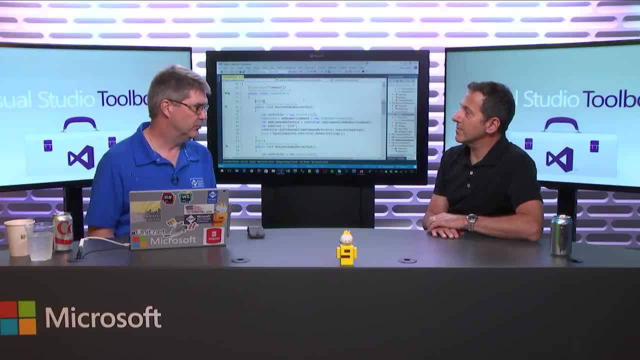 So when you and I are talking about building something, building a house or remodeling the studio- you would say I would like a door here, Right, And then later you'll have to figure out: does it need to be soundproof? 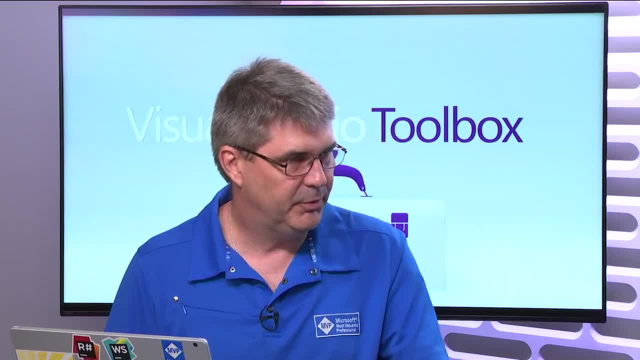 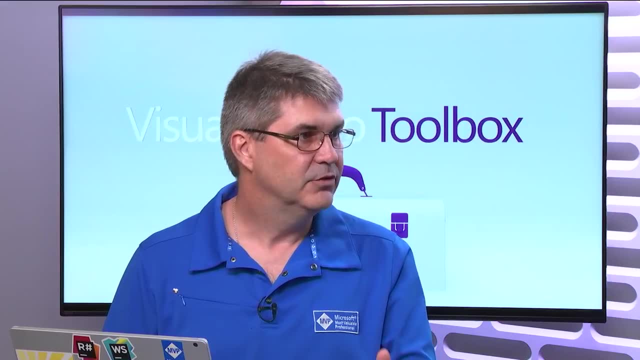 Should it be able to lock. Those implementation details come out later. Okay, But you and I both know what we're talking about when you say I want a door there, Got it. Software design patterns are the same thing. So instead of going into great detail when we're discussing how 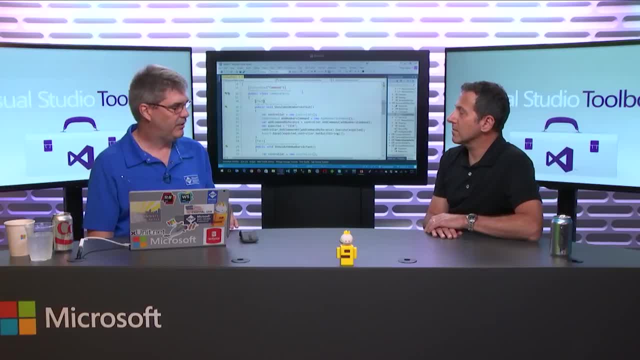 we're gonna implement a particular feature. if we could talk about it in the design pattern level and figure out how we're gonna solve the problem without getting stuck in the weeds, then you and I could both agree that, for example, we need to build an e-commerce application and 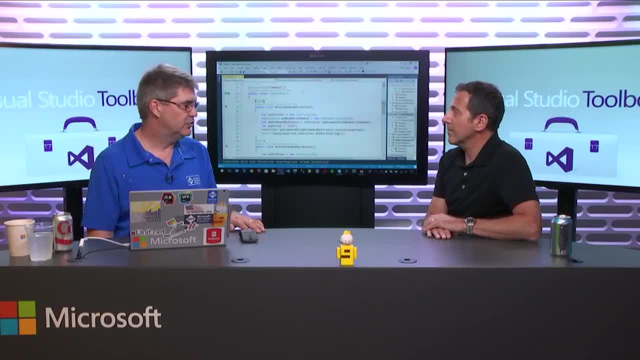 the main part of that application should use the command pattern to shell out to the specific implementations of charging a customer, picking, inventory, packing and shipping, Okay, And we say, great, that's perfect, Let's use a command pattern for those. and 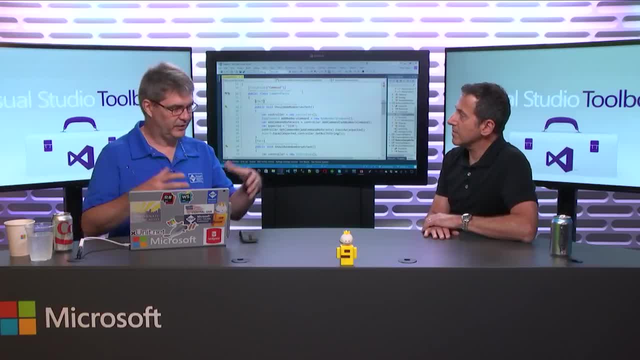 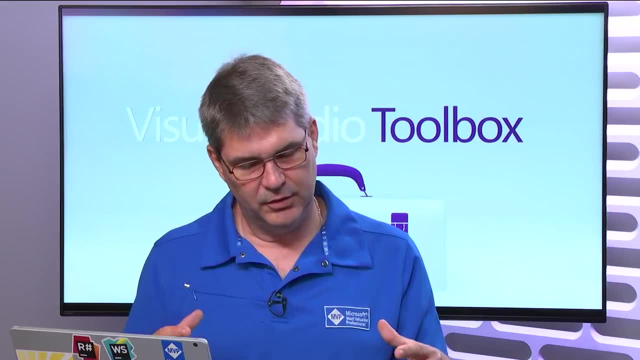 then we go off our separate ways and start working Now. is that the only pattern that we're gonna use? No, we're probably gonna use more, But the goal is to be able to communicate, solve problems that have already been solved and make it easier to support. 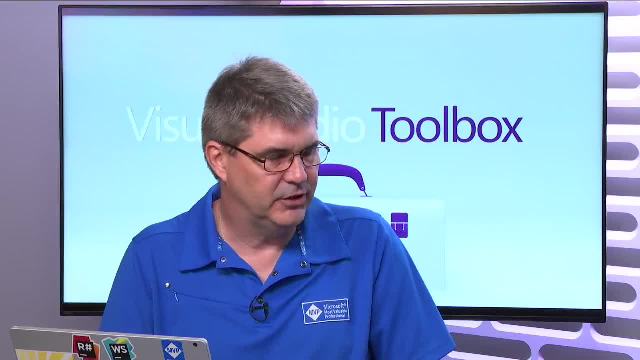 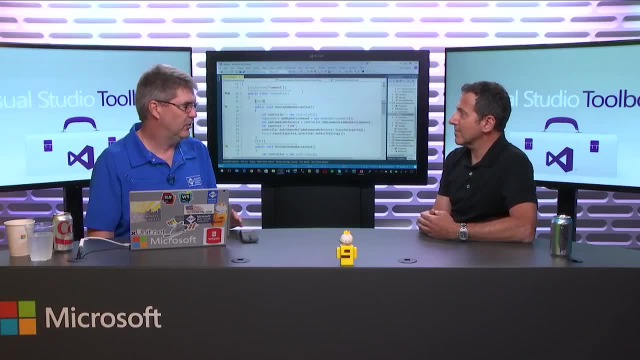 Years ago I had gotten to take a vacation in France, and this was long enough that we didn't have cell plans over there, right. So it was a fortune for me to talk on the phone, and I had a lady who was backfilling for me at a customer. 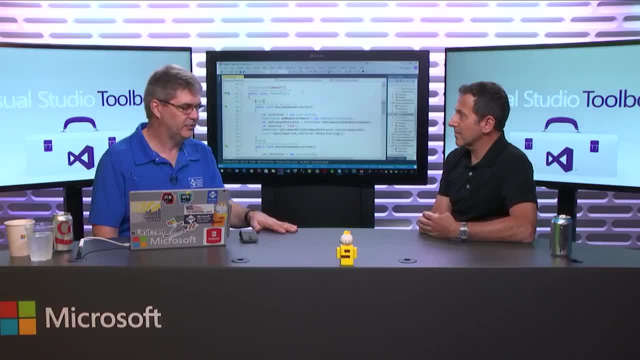 And she was charged with fixing a production bug cuz I didn't have enough unit tests in place. And she called and said: I don't understand what you're doing here on this form- and I'm looking at my watch going my gosh. this is hugely expensive. 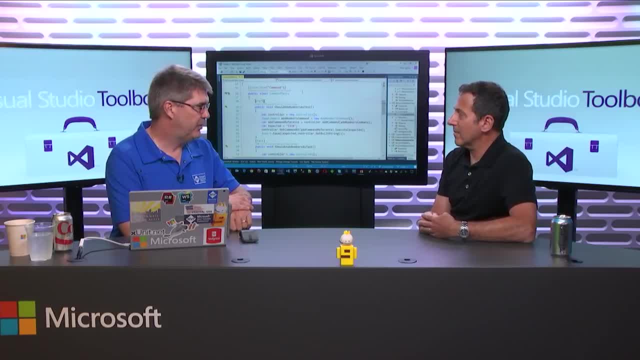 And I said that screen- I used a strategy pattern for that- And it was like a light bulb went off. She was okay, bye, have fun, and she hung up And then it's like she saw the lady in the red dress. 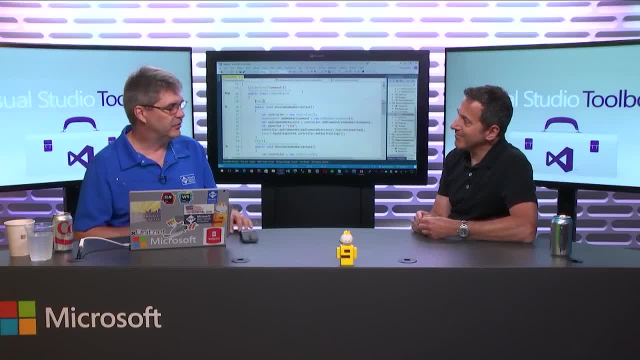 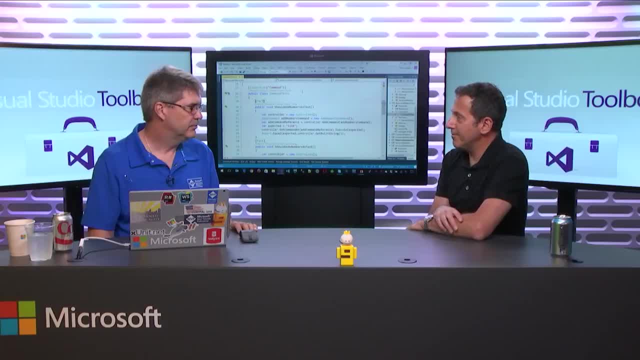 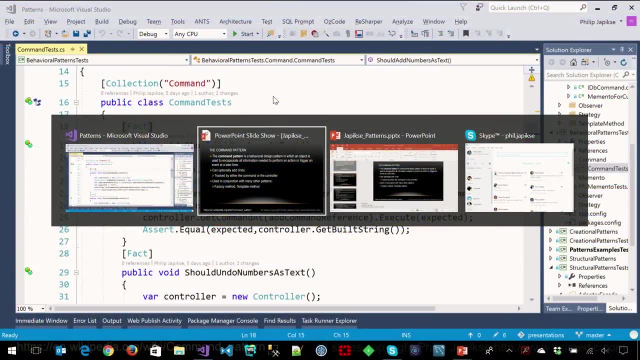 It's a lot of work Standing on the shoulders of giants. Okay, cool, Does that make sense? It does, Okay, so let's talk about the command pattern first. It's probably one of the easiest patterns out of the entire book. 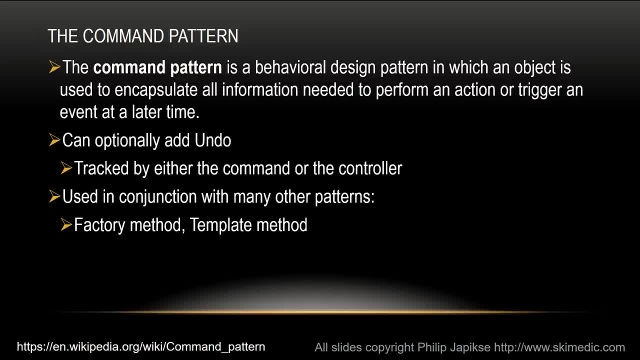 So the command pattern, and we'll do this through all of them. We've got the Wikipedia definition I want you guys to have- or you guys to have, sorry- And then we will actually go into code and then talk about practical uses for it. 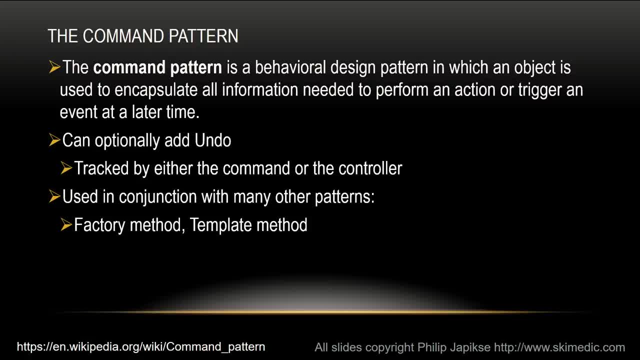 But the key thing with the command pattern is it's used to encapsulate the information needed to perform an action or trigger an event at a later time, So let's just stick with trigger and action. You have a remote control at home, right? 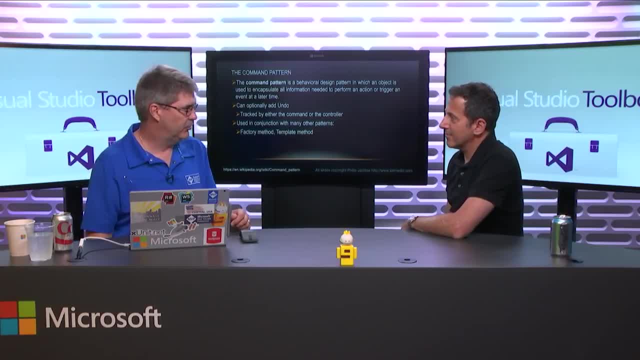 Sure For electronics, Mm-hm, And you and I are probably of the age that our remote controls have a VHS button in addition to it, maybe a DVR button, DVR, CD, SAT, Yep, Exactly, Yeah, all those. 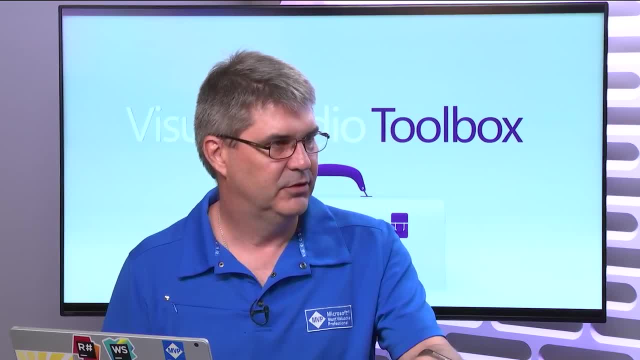 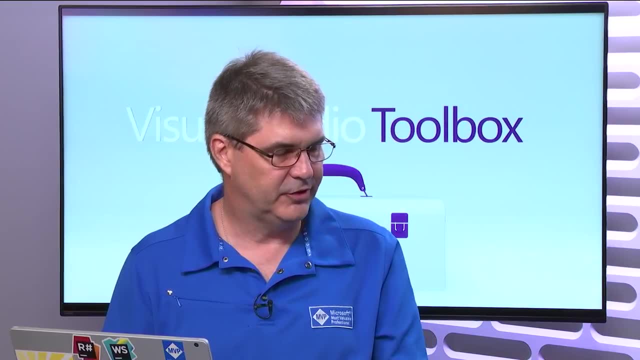 So the remote control knows nothing about the DVR player, the satellite, the. you know the device, the device that you're using, Yeah, The cable box, the TV. It just knows that when somebody pushes this button, it sends out a command. 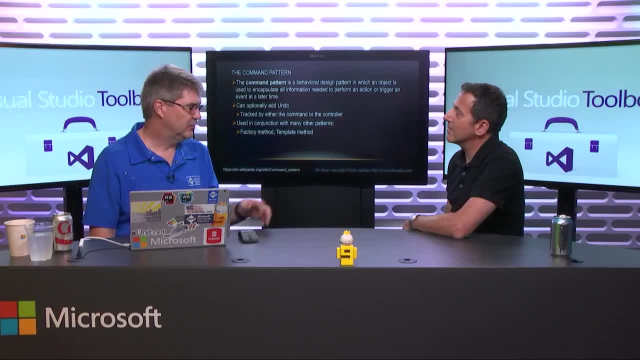 Right, And for most electronics that command is a bit flag: If I'm on, turn me off. If I'm off, turn me on Right, Mm-hm, And you have to program the remote control for your specific make and manufacturer. 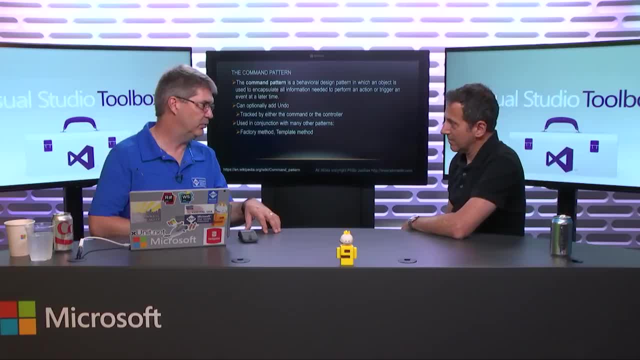 You don't have a button for every single manufacturer or every single model number, you got just one button and you program that. So the command pattern works the same way. You've got this controller, which could be remote control, could be a factory method or a template method. 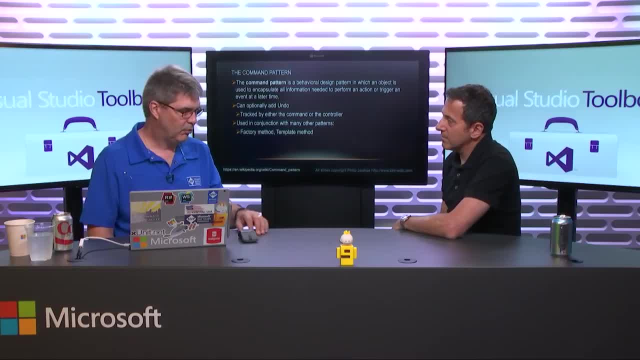 which are patterns we'll talk about later in this series- Where it says: charge the customer Mm-hm And that is the command. You write the code. it charges the customer. it's gonna ask them if they need Visa. 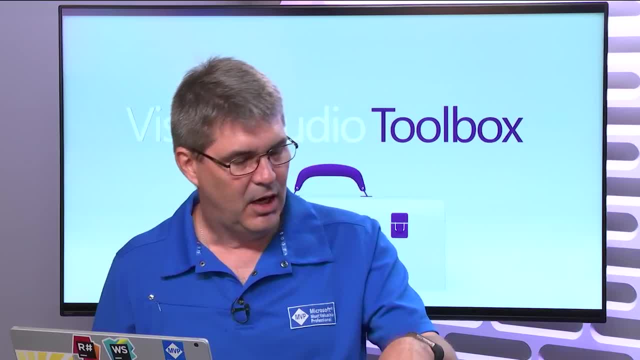 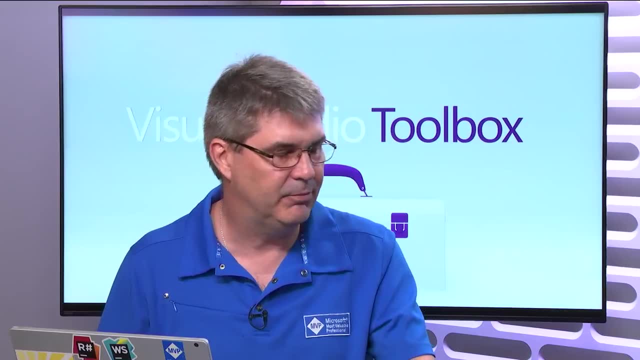 you know MasterCard Express. however, they're gonna do it right, But I in writing this main method that calls the command to charge the customer. I don't need to know any implementation details, Right, Right. So that's the key thing. 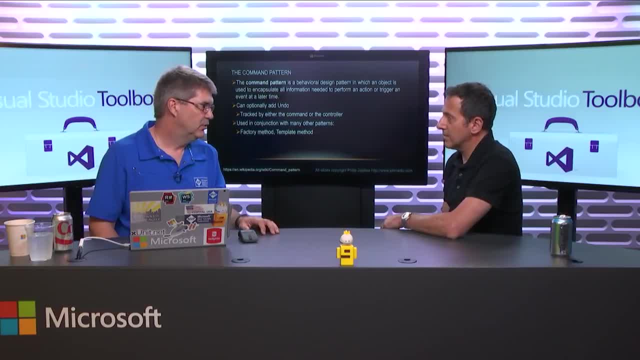 Now there's an optional aspect of command. it's the undo. So with the remote control, it's not really a good example for undo, because you just push the button again and it turns on or turns off, Sure, But a great example of the command pattern with undo is. 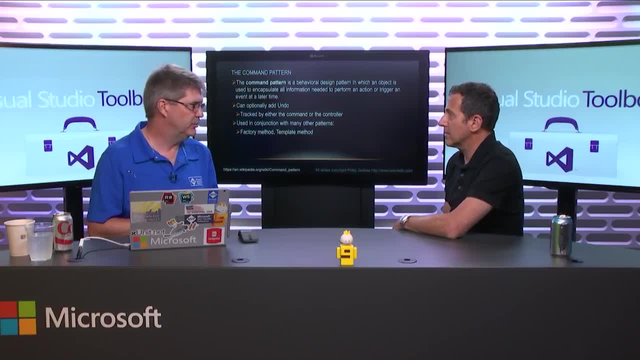 you know the most famous keyboard combination that all developers use, which is, of course, Control-Z, right, Mm-hm? I didn't mean to delete that Control-Z. That's a command being set from the keyboard that goes into Visual Studio, or. 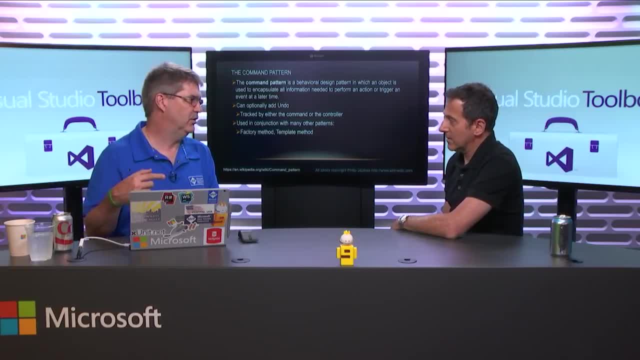 Microsoft Word or whatever, and reverses the last action done Right. So it's keeping track of what you did and then calling an undo on that, And so you know it's an optional part of the command. A refund to customer is probably a different process. 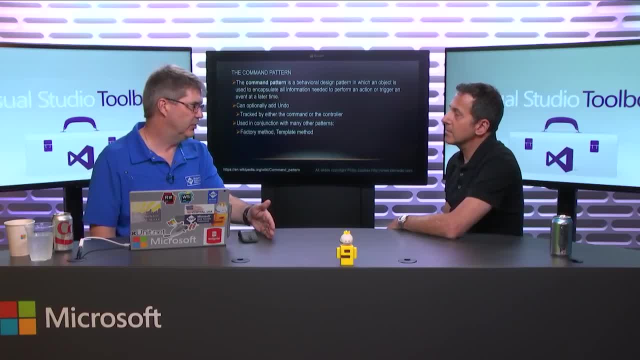 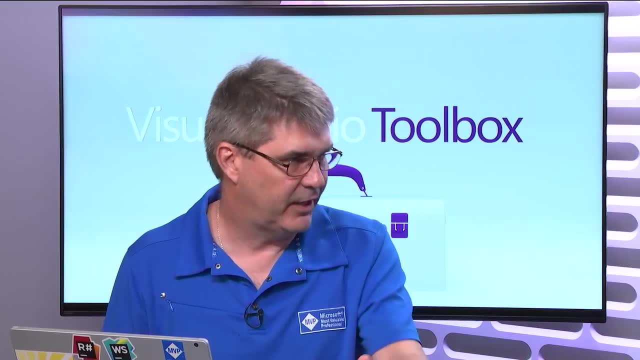 Right, So the charge to customer might not make sense to have an undo. but to pick inventory, to have an undo probably does make sense. Yeah Right, Because you can put the inventory back right where you found it. Right, Right, So let's look at code. 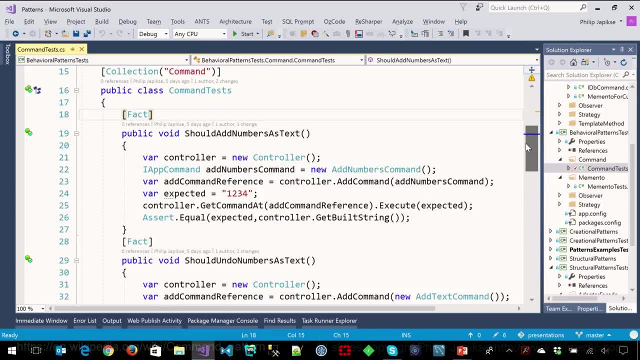 And, as we discussed in the TDD episode, I always write unit tests, or try to. If I don't write unit tests before I write my code, I feel a little dirty. It doesn't mean that I never do, it just means sometimes I need to take long showers to clean myself up. 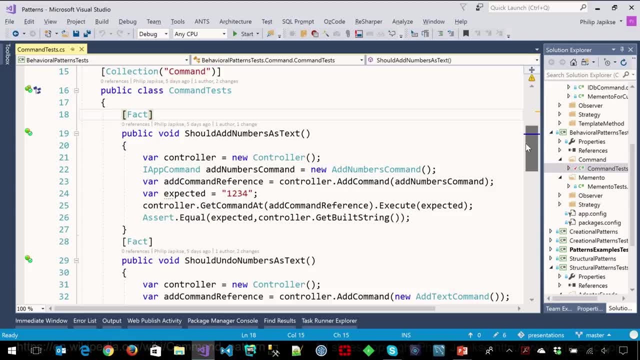 But I find it much easier to describe how something behaves by using a unit test than trying to write a whole bunch of domain-specific code to then show this one particular aspect Right. So here I have a controller. This would be like my remote control. 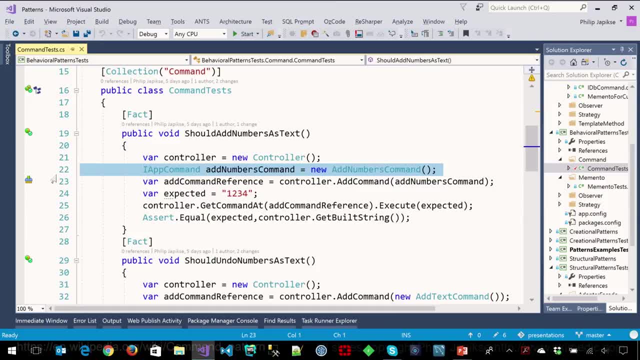 I have an interface that represents a command, and in this case it's an add numbers command. Now, this is a very trivial example. I basically have a string builder that I am either adding text or numbers to, and then I have the option of undoing the last command. 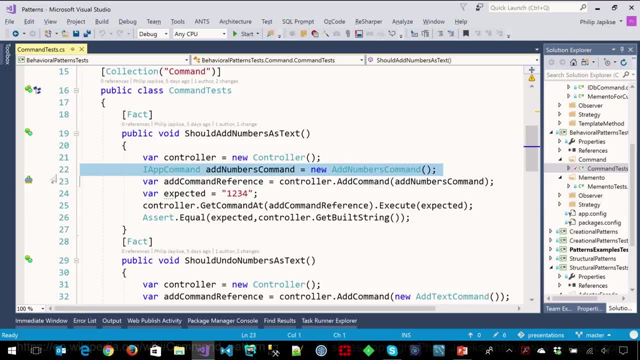 or the last series of commands. Okay, Is this something that you would do just like this in production? I hope not, because it's like writing the Fibonacci sequence, right? We all learn it in school. I've never been paid to write the Fibonacci sequence for anybody. 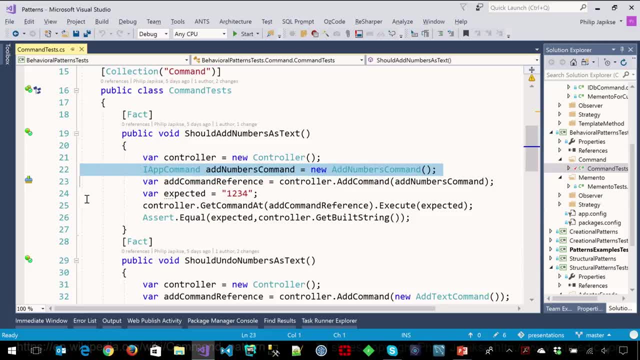 So it really is just sample code to demonstrate to principals. The controller has to know about the commands, right, There's some way I have to be able to push that button. Okay, This is you programming the remote by using that real fine print on the big remote control sheet to say: 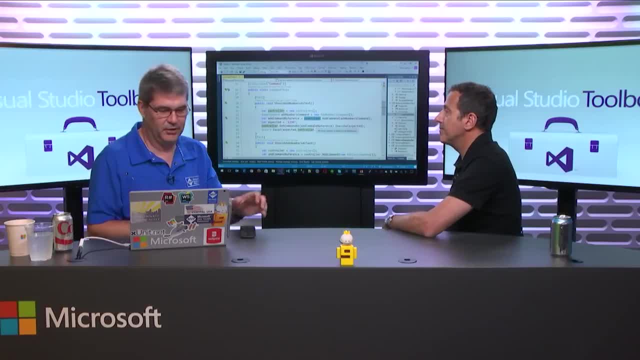 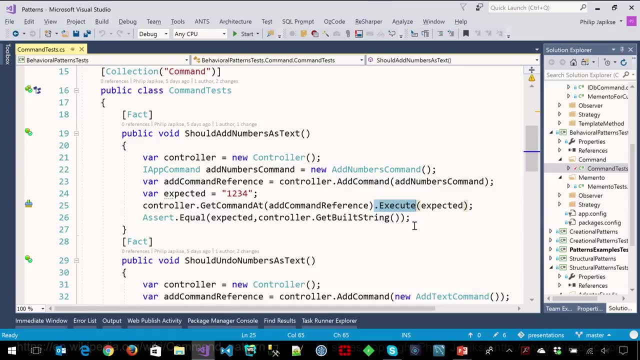 I have a Vizio TV right And you push in the right numbers. I then execute the command, passing in the value and that's probably not the best variable name for it. Okay, But the three hardest things in programming, don't you? 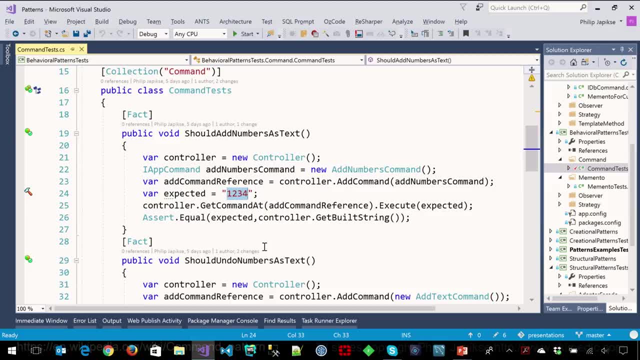 It's off by one errors and naming conventions, Right? So then I just check to make sure that the string builder is returning 1,, 2,, 3,, 4, right? So it's very simple. I'm basically just putting things on the end. 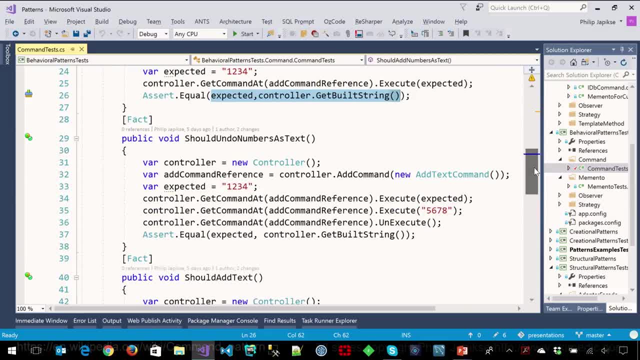 But let's say, I want to undo that and we'll look at the code and how all this works shortly. So we want to undo same thing Now, before we move to undo, where's the command pattern in that? Oh, good point. 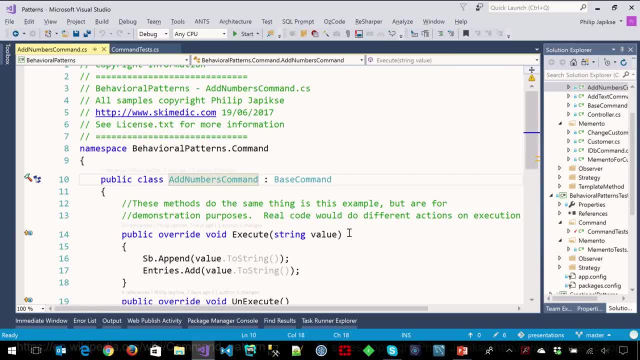 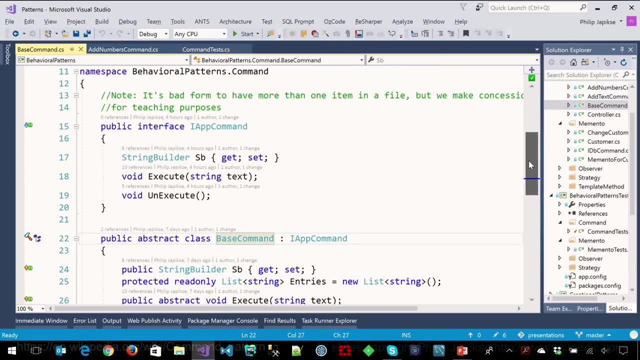 I was going to show you to undo, then we're going to go into it. But you're probably right, This is a better order. So I have a base command which implements the I command. Now I do have comments in here all over the place. 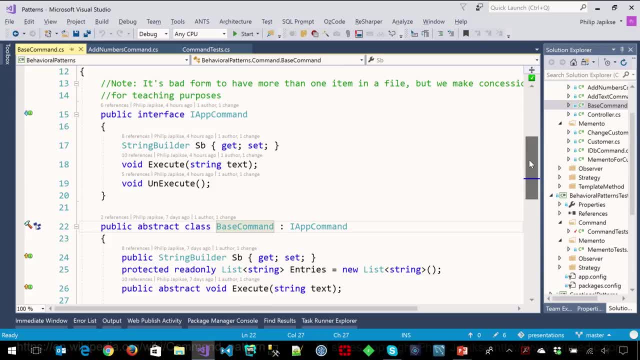 It's bad for them to have more than one object in a file, But for teaching it just makes it easier. so it bounced back and forth. So my I app commands- and I just made up that name, because command I command is actually taken by WPF. 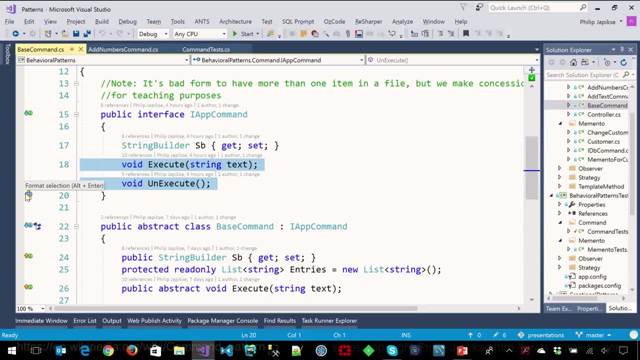 I have an execute and an unexecute, And the execute takes in string- This is what we're adding- And unexecute doesn't take a parameter because it's just saying unwind the last thing I did. right If I had to pass in a parameter. 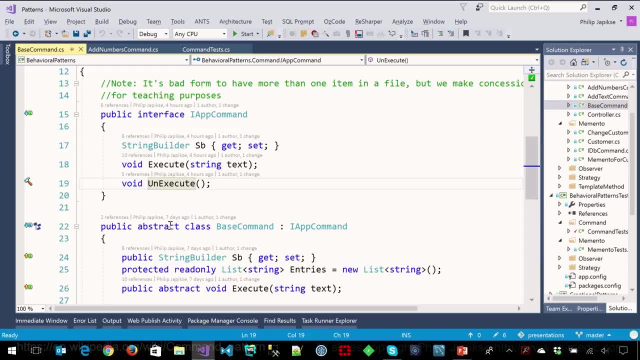 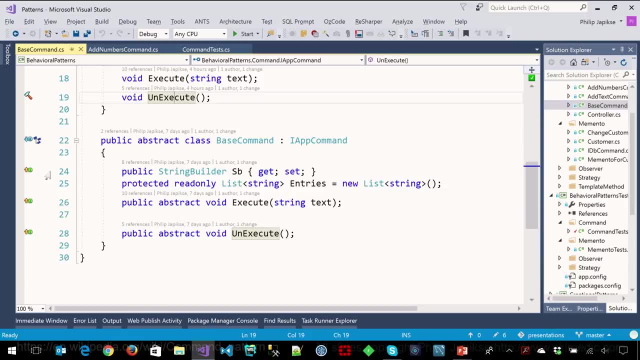 it would be like Control-Z, requiring me to type in what I wanted to undo in order to undo it. So I have a base command, and the reason I have a base command again for my silly example- is to keep track of the string builder. 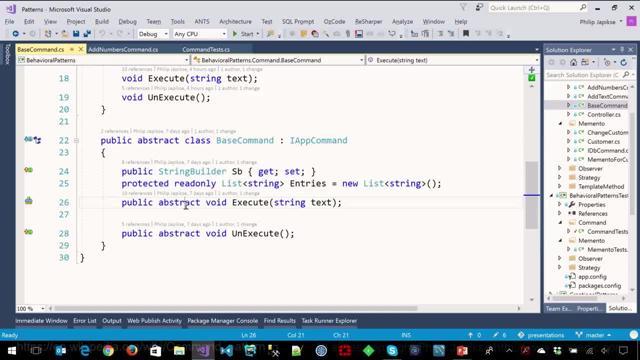 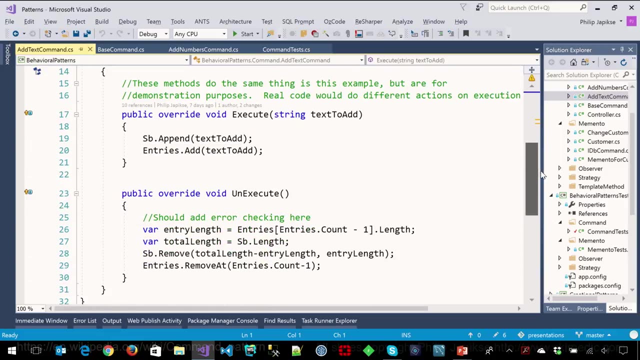 Okay, And then I just make the execute and unexecute abstract. So my specific implementations of the commands have to implement them. So my add command or add text command, I have an execute which just appends the text to the string builder. 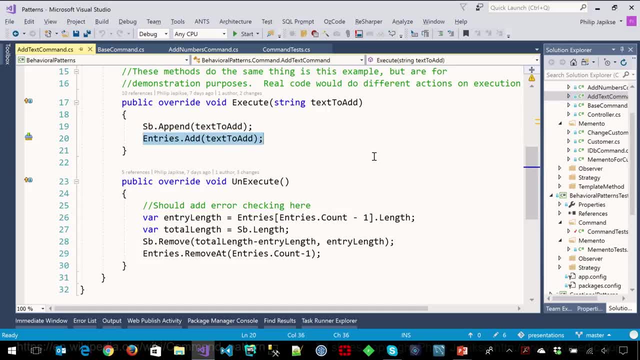 and then adds that text to a list. but where I'm tracking the items I can undo It's the same as in Visual Studio. you have 20, by default I believe it's 20, undo operations you can do Right. 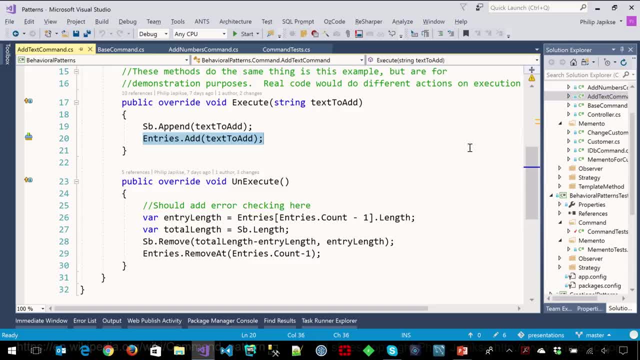 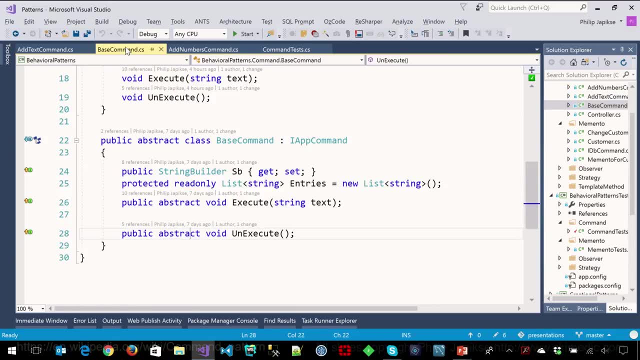 You can change up buffer, then it uses more memory, things like that. Now you'll notice. let's go back to the base command, Because I am keeping track in the base command, but not like a static command, the undo only works at that particular command level. 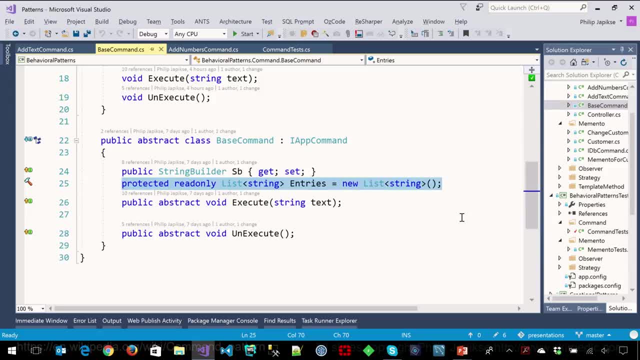 So let's say I have an add text command and an add numbers command and I add text, and I add text, and I add numbers and I add text. Then I want to undo the add numbers. Yeah Well, guess what? There's a bug in my program. 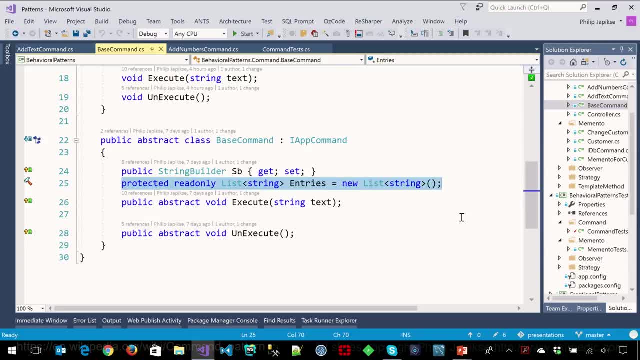 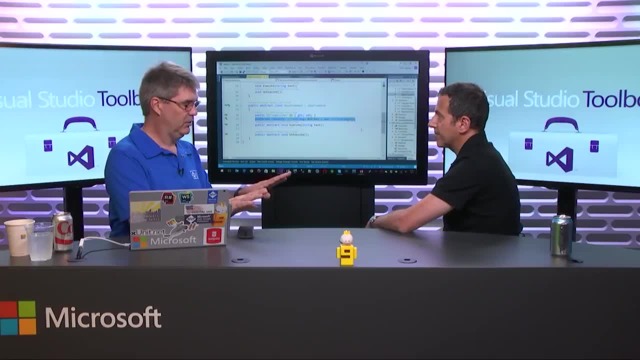 because it's going to undo the last operation, which was the add text. Then when we talk about memento, next in this episode, we'll talk about where we can restore states to a previous point in time. Okay Right, So we have to unwind. 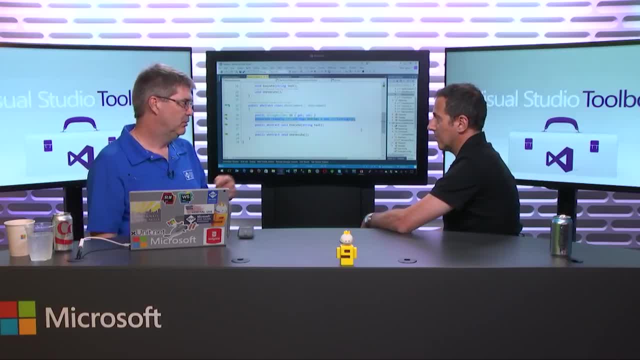 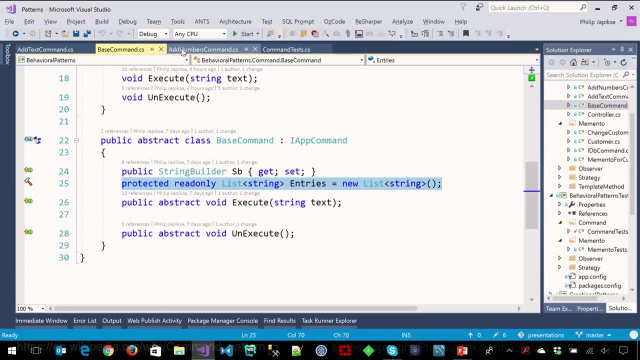 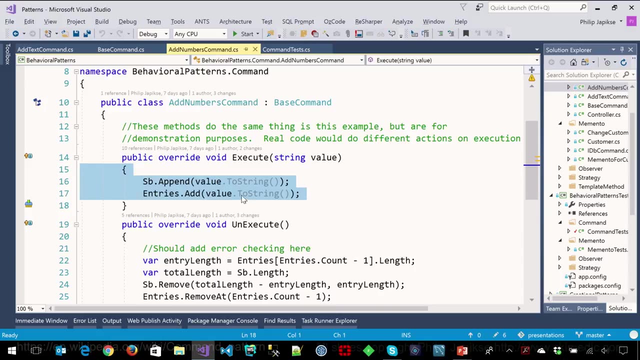 the stack. in this style of implementation, one at a time, We can't jump to a previous point in time. Okay, Does that make sense? Sure, Okay. So here we have added a value to the string builder. We've popped that string onto this stack of undo operations. 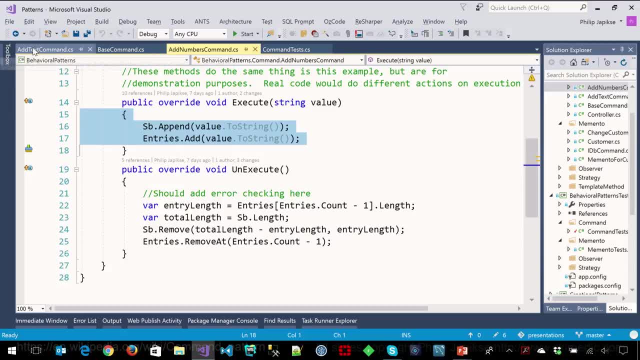 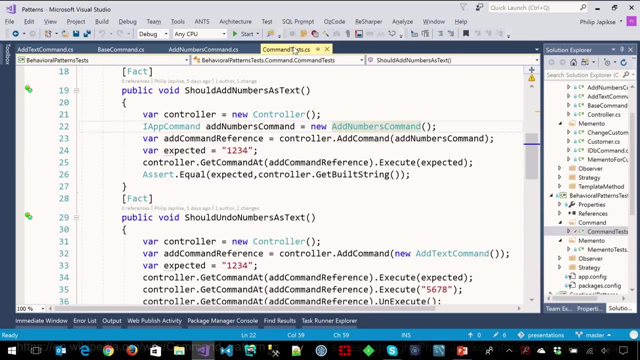 Right. So now, if you go back to the code, Which code? The original? that code there? Yeah, The fact that you are calling controlleradd command, is that the command pattern, Because this code doesn't know the implementation of what you're doing. Yes, 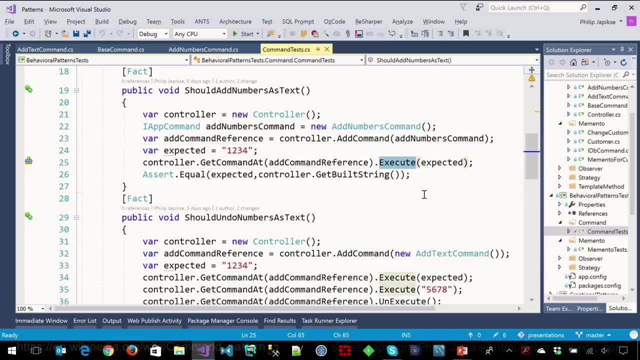 So The execute? There it is. The execute is the implementation of the command pattern, Got it? What this is doing, this is you programming your remote control for your Vizio TV Right? So the execute, So the fact that you have encapsulated this, 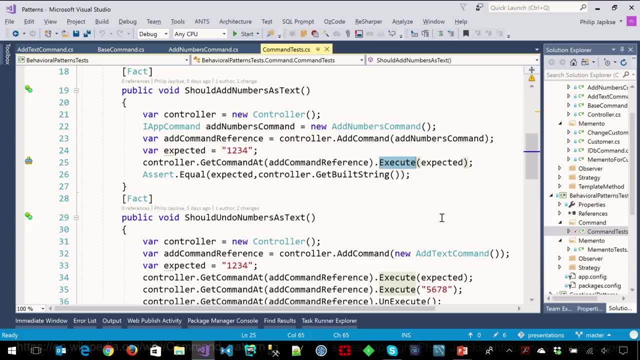 you've taken that code out of this method and put it into a class. I've completely encapsulated all of it, right? Yeah, So the controller doesn't know about the string builder. Right, I could be adding stuff to a file. 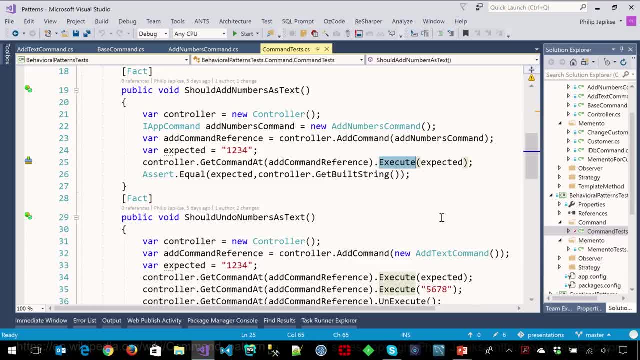 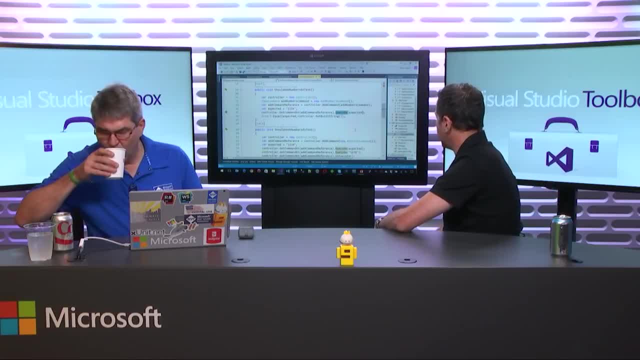 I could be adding, pushing stuff into a database, Any number of implementation details You've in this code. you've told your assistant to execute. This is basically the equivalent of having staff. Yes, Right, Yep, Go do something. 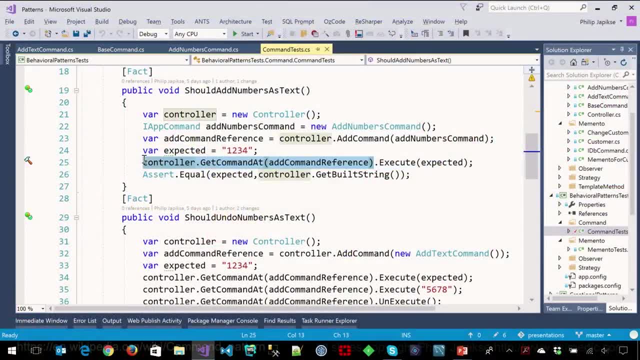 Go execute, Go do something. I don't need to know how you do it, Get it done, Just go do it, Get it done. And I may want to know what the results were. Did it succeed, Did it fail, Or you know? 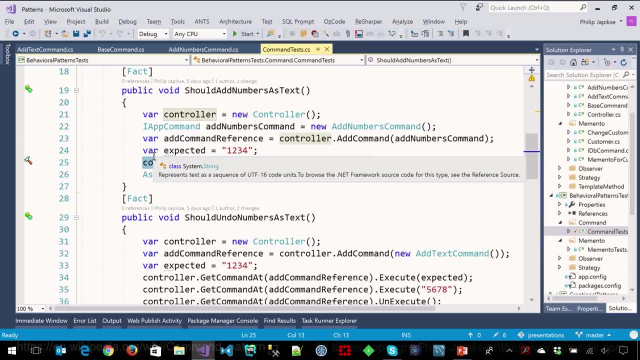 go do something, tell me the results, but I don't need to know how Right. That's the command pattern Exactly In a nutshell. Okay, And this code here that is just picking which button to push Right On the controller. 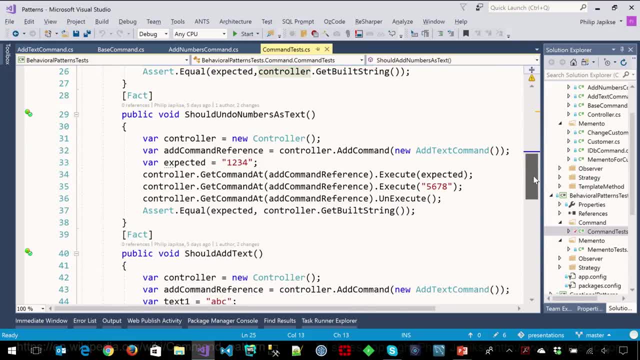 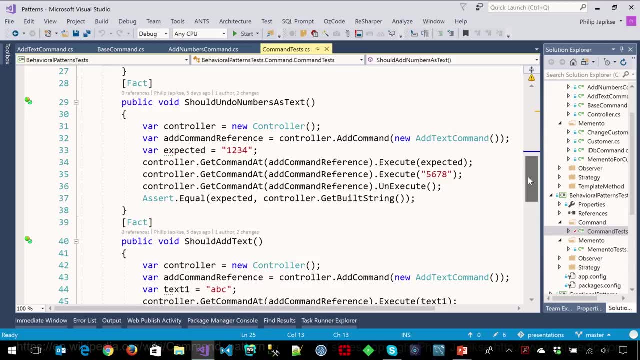 Yep, Now you might also want to tell your staff: ah, I told you prematurely to do that thing. Can you go undo it? Right, Right. And again, you don't care how, You don't care how you do it. 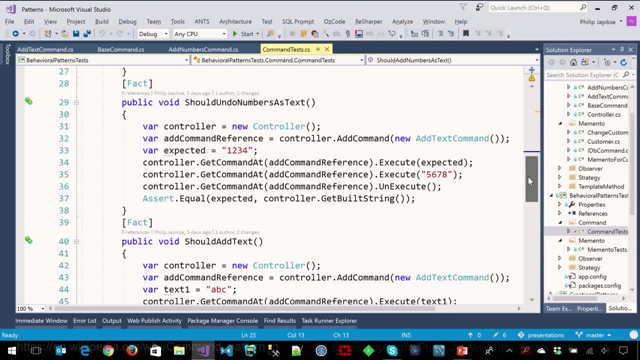 You don't care how you do it, You just want them to go away and report back later. Yep, I've undone it. Call the fixer, Call the fixer. So this is the exact same thing, pretty much, Executing: adding the one, two, three, four. 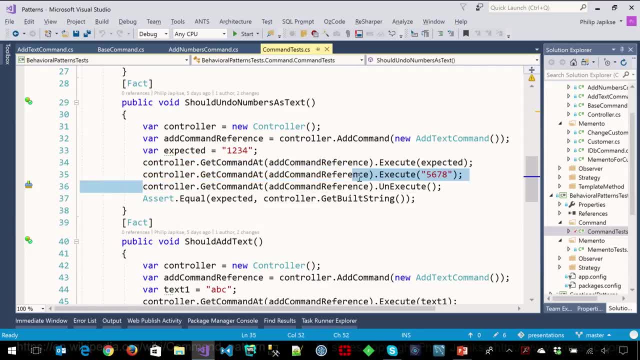 then I add a five, six, seven, eight. I then call unexecute, which unwinds at five, six, seven, eight, addition to the string, And then I verify that the string that I get back is the one: two, three, four. 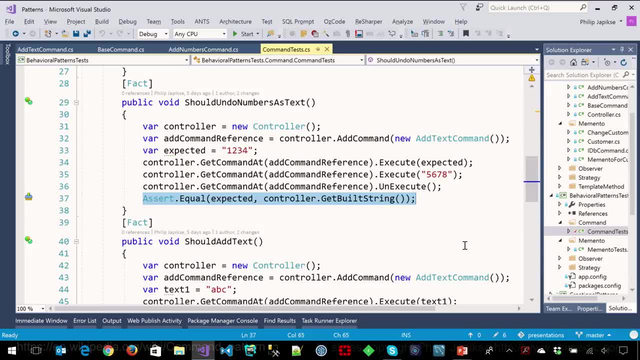 which was the state prior to executing that command that I undid. Right, Got it. So that is like I said. it's a really simple pattern to code Mm-hm. But there's, as we were discussing over lunch. 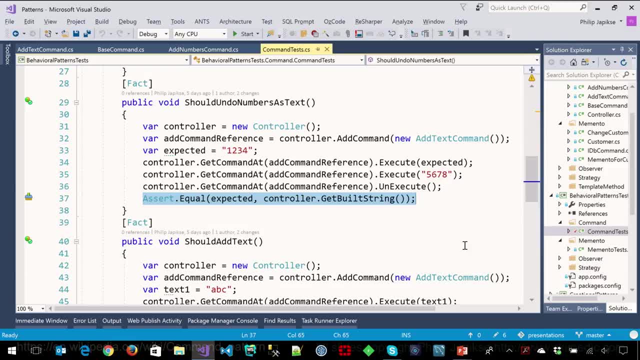 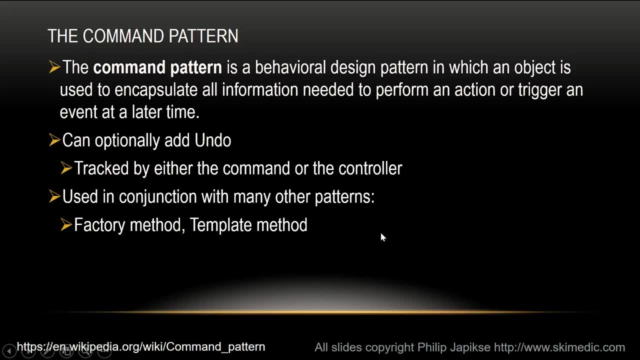 there's lots of implications about, well, is this really the command pattern, or is this not the command pattern? So before we go into the memento, let's kind of come back and redress this. Yeah, so let's use the example we were talking about. 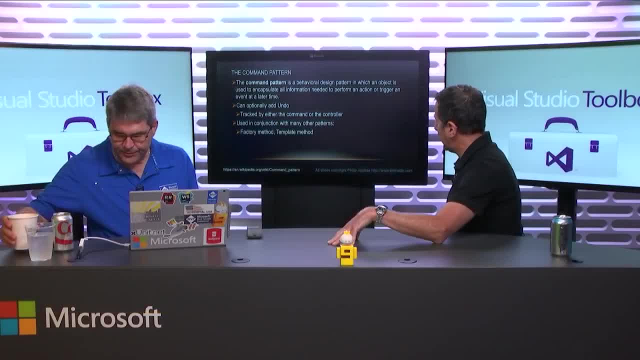 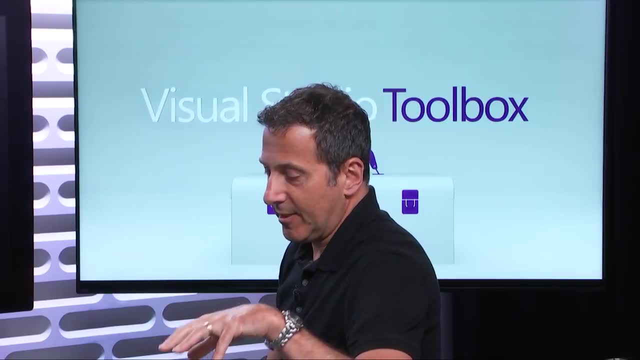 I'm writing a weather app- Mm-hm Right- and I've got a UI. I've got a text box or it could be a drop down, Some way of identifying the city button to get the weather, and then one or more labels to display the results. 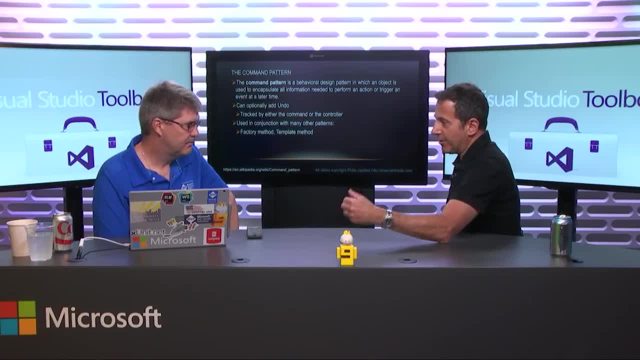 Okay, In that button I could put the code to call the weather service and do all the manipulations. I could put all the code in the code behind. Okay, let me stop you there. Yeah, Because we did this for years with VB. 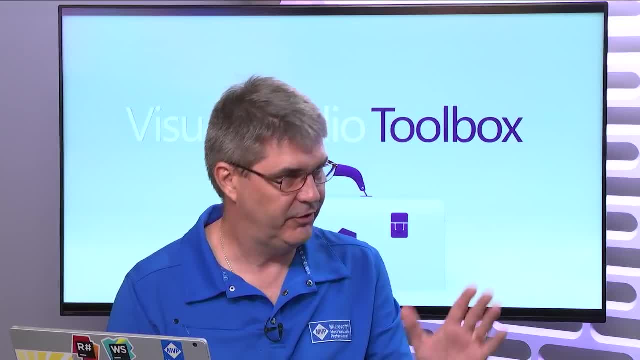 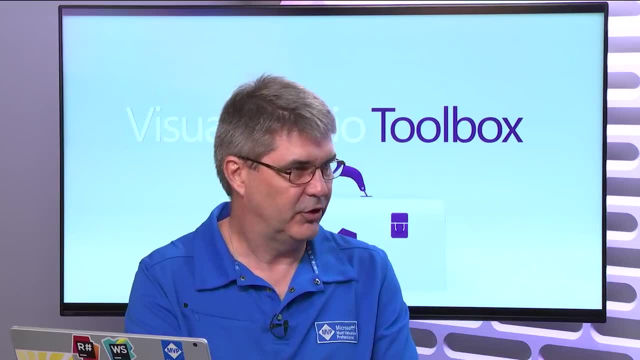 Yeah, Right, And I'm not knocking VB, it was just kind of how we did things right. You have a form, you double click on the button, you get the click event right there in the code behind and you started coding stuff. 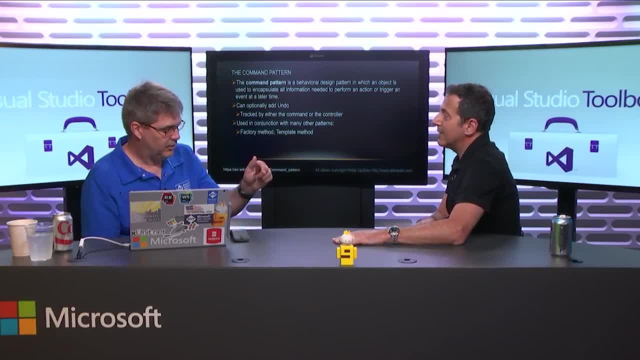 Right, you put in the entire implementation in there. Okay, now push the button. calls the weather service label gets updated. everybody's happy, Right? Then that weather service goes out of business. Yeah, Now what do you do? Or you wanna reuse that code somewhere else? 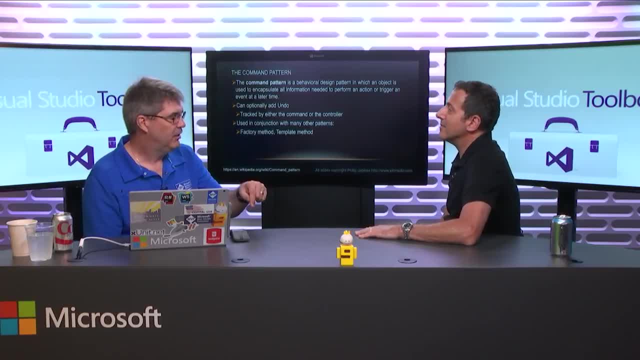 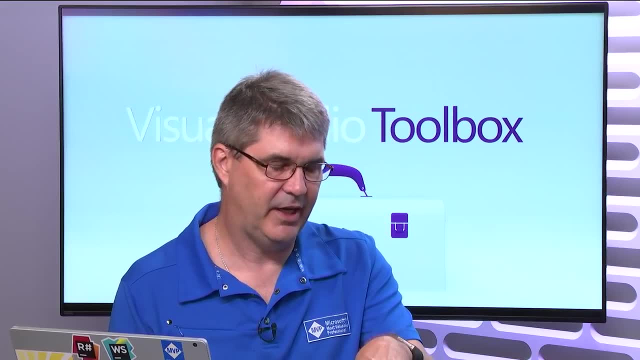 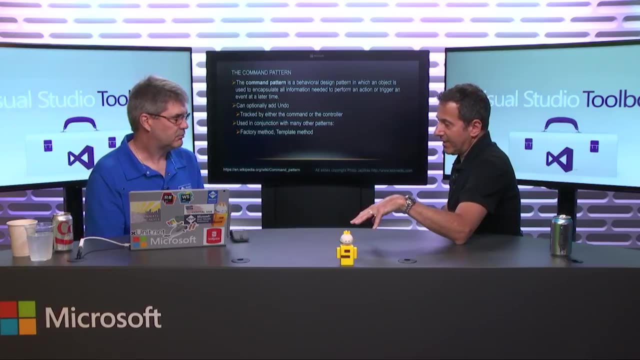 Or reuse that code somewhere else. Right, yes, Either way, I have to go now and either clipboard inherit that code somewhere else, or I have to change that production code because I tightly coupled the command to the implementation. So instead I create a weather class, weather service class. 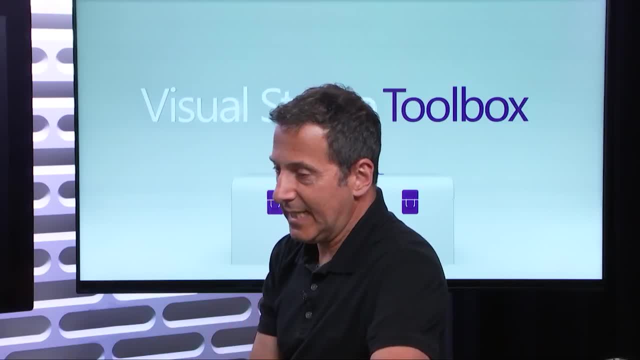 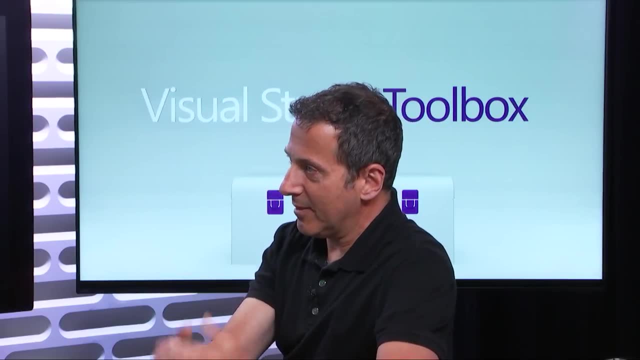 I usually call mine weather service, cuz it is essentially a service. Yeah, And then in the code behind var, weather equals new weather service. Okay, WeathergetWeather. passing whatever's in the text box Labeltext equals whatever that thing returns. 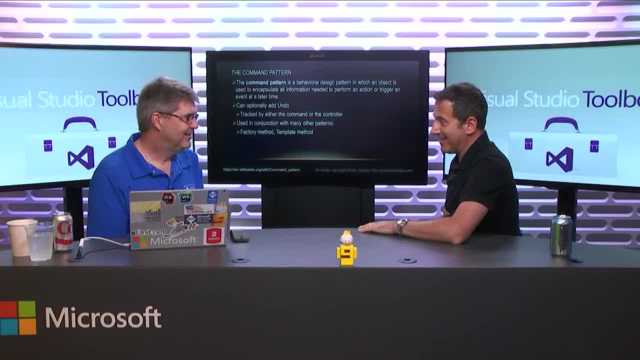 Yes, Is that the command pattern? It is, but it's making me twitchy Because I'm not using an interface. Because you're not using an interface, Do I have to use an interface for it to be the command pattern? You do not have to use interface for the command pattern. 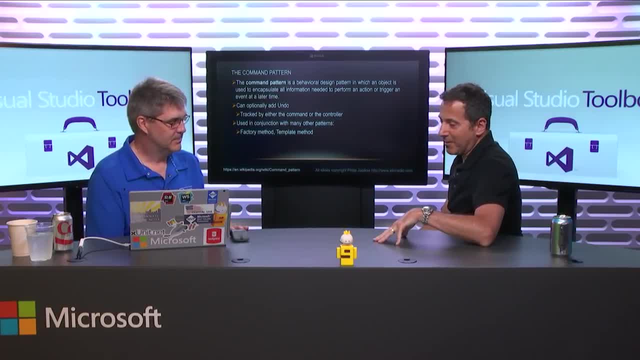 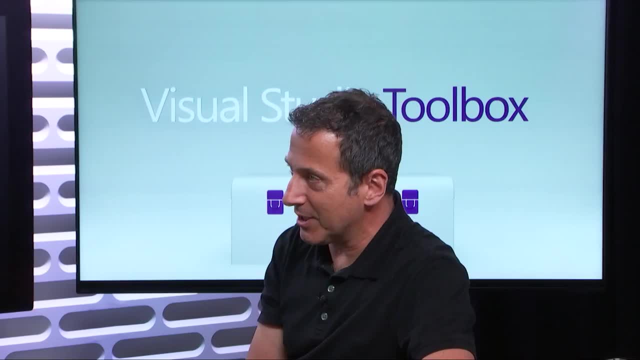 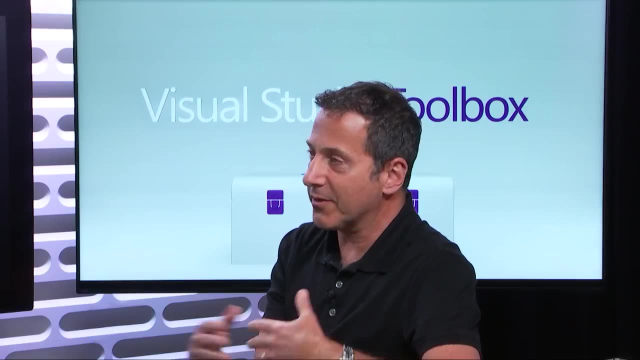 Okay, now the fact that I should then think about- for reasons we'll talk about later- when we get to things like the factory method, I should do more encapsulation. What happens if the weather service changes right? What happens if I want to have an online versus offline version for it? 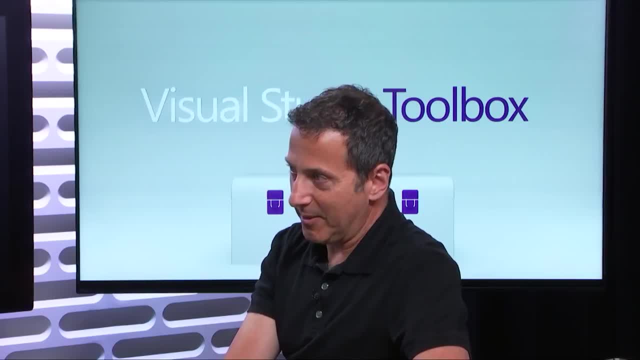 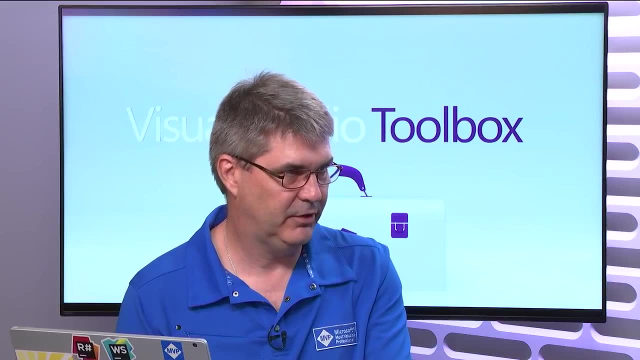 There are all kinds of good reasons why I wouldn't stick to that. Well, let me go back to our previous episode. Mm-hm, If you say var foo equals new weather service in your button clip, Mm-hm, How are you gonna test that the button is actually calling the weather service? 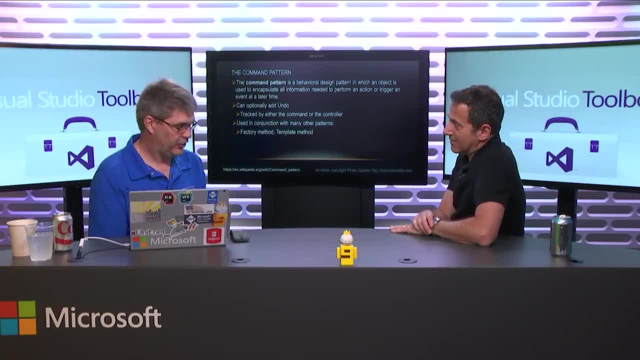 Let's say you're on an airplane and you have no internet connectivity- Mm-hm- And you push that button, Yep, And the app just hangs. Where's the problem? Right? so then what I'd have to do is I could go into my weather service and 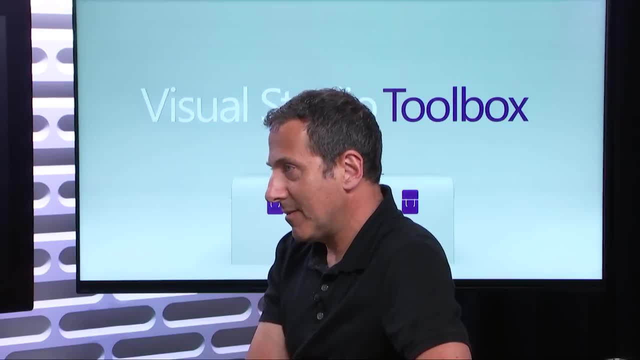 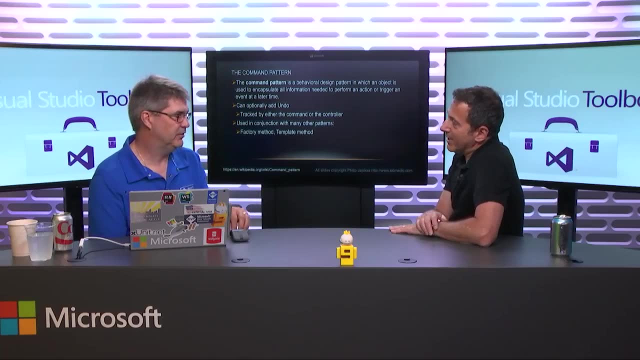 have that call an interface, but that's just kinda kicking the can down the road. Or I probably should do that in the button, Or the button talks to an interface, Right, Any time the phrase that commonly gets thrown out there. 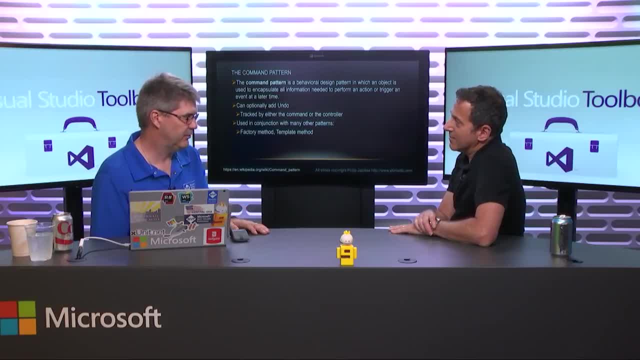 and I think it's a good one. new is glue right. Good friend of mine, Steve Smith, who's really really deep in the patterns and code quality, uses that phrase a lot And it's true. Once I say var foo equals new var, then I am stuck to that implementation. 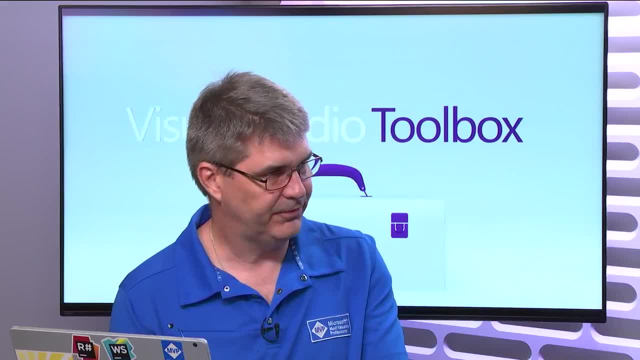 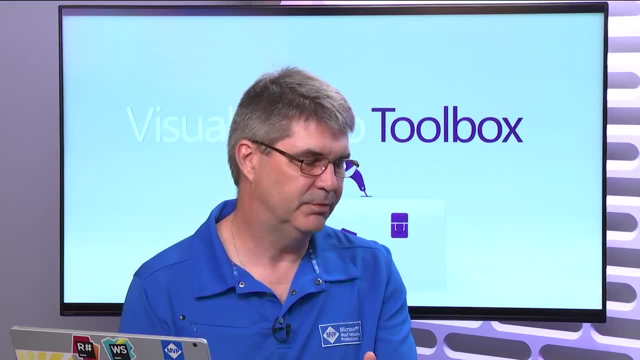 Right, Or I have to go in and change code. Yep, If I code to an interface, then I'm not dependent on the implementation Mm-hm. So let's go back to testing that. We showed you how to use mocks. M-O-Q, the framework to create a mock. 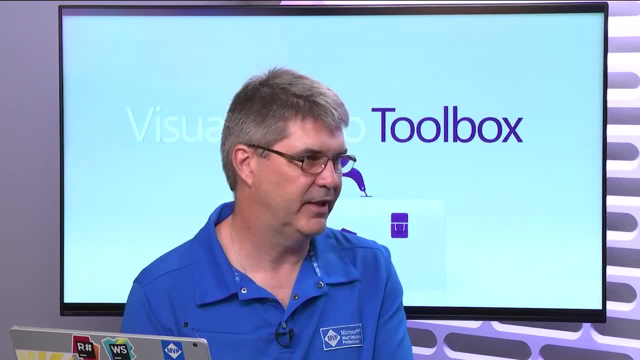 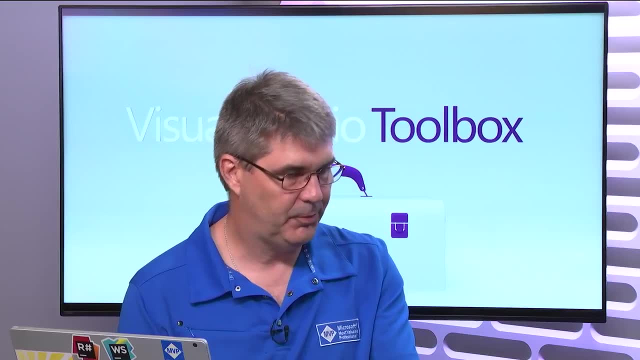 Mm-hm And then set up a expectation that a particular method gets called Right. So we can set up a test that where we pass in a mock Of the iWeatherService, set up that it calls getWeather with a particular string or 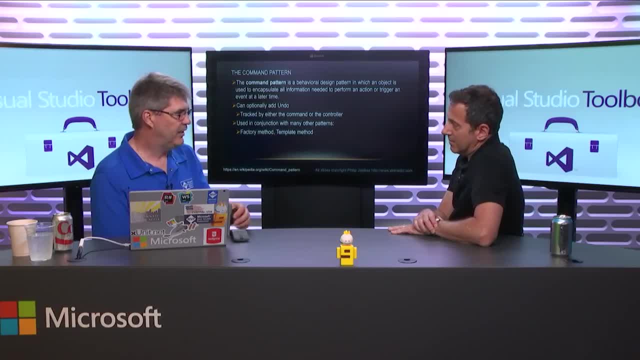 any string and then we can verify it was actually called. So then in that button click method we could write a test for that and say: does it call the weather service, yes or no, with the correct parameters: yes or no. 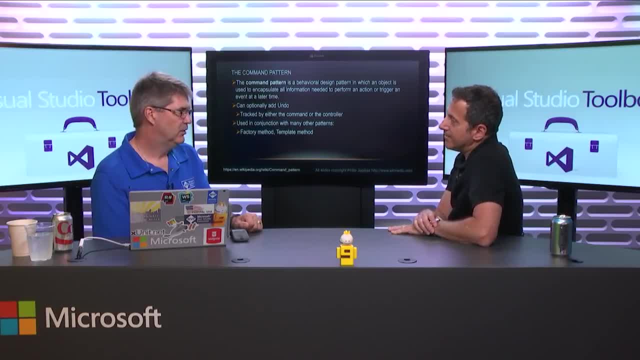 And if it does, we know we're good, right, Yep. So it just further encapsulates code, making it single responsibility, right, Right. And it just enables all kinds of options that you don't have otherwise, Whether or not you do that. 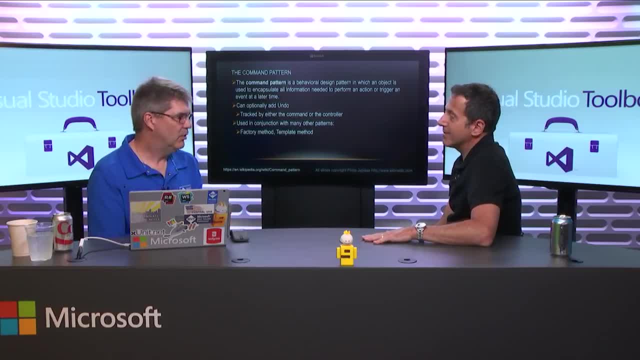 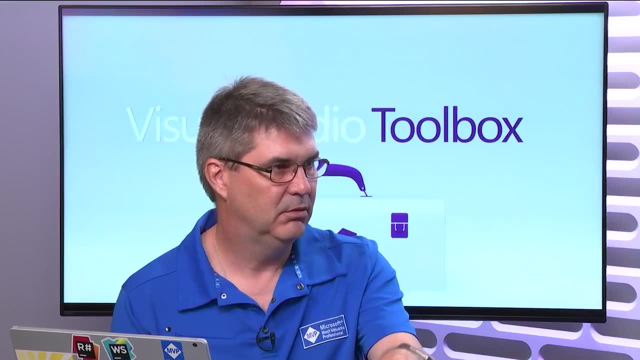 Whether or not you do that, it's still an implementation of the command. It's still the command pattern. Okay, What we have done is we've encapsulated just what it says here. Right, We've encapsulated all information needed to perform some function. 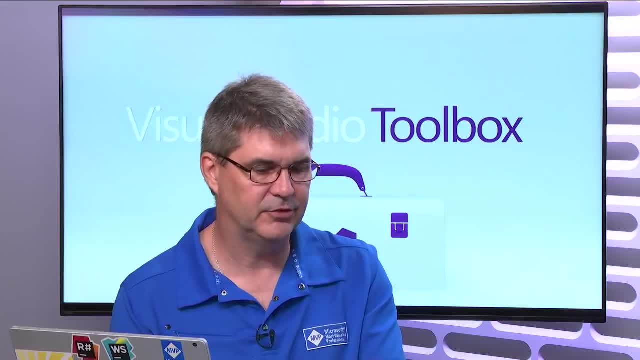 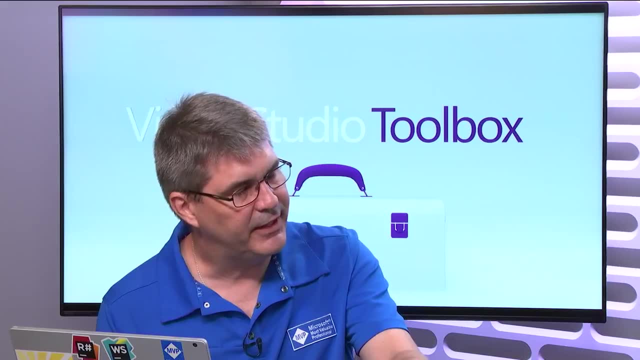 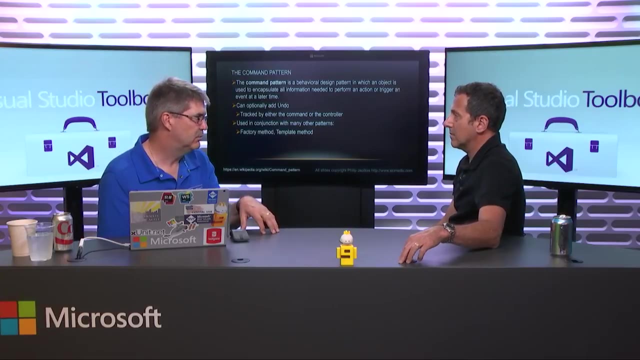 Okay, Now, sometimes people will look at it and say it's really only the command pattern. if the command that you're calling manipulates some object, Like so saving a record to a database versus going to get the weather right Or making a change- 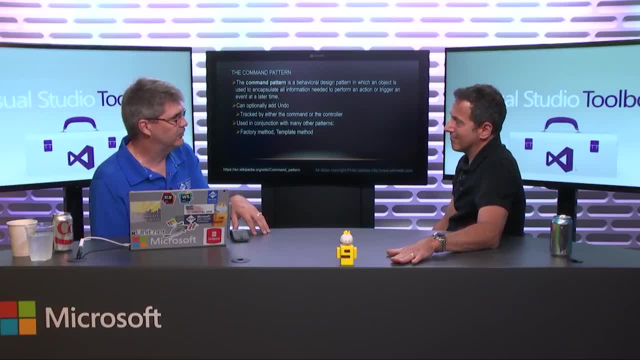 I'm not saying I agree with this. I have had discussions with people at conferences. Mm-hm, And that's the beauty of command patterns, right? It really is just a guideline Right To a problem that's been solved before. 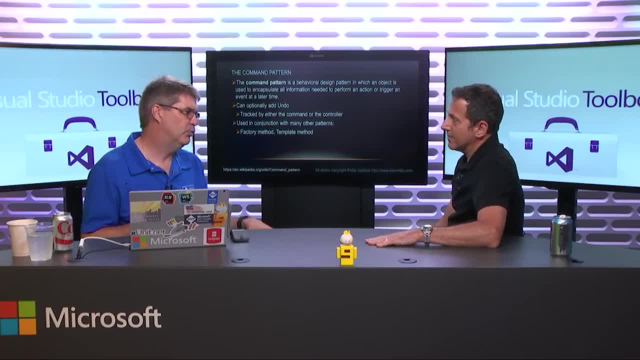 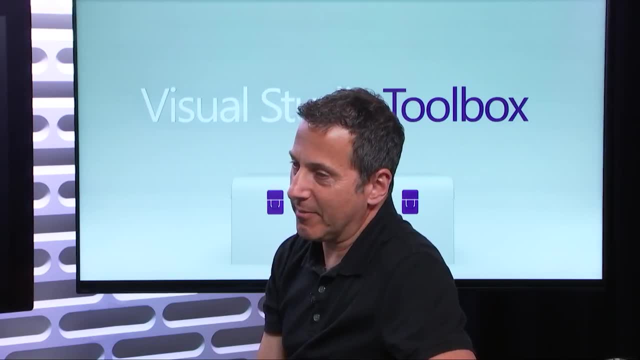 and you can implement it how you want. Right? It's a bit like the pirate code: It's more of a guideline than an absolute Right, And then it becomes just a question of implementation. True, Now you're talking about what? 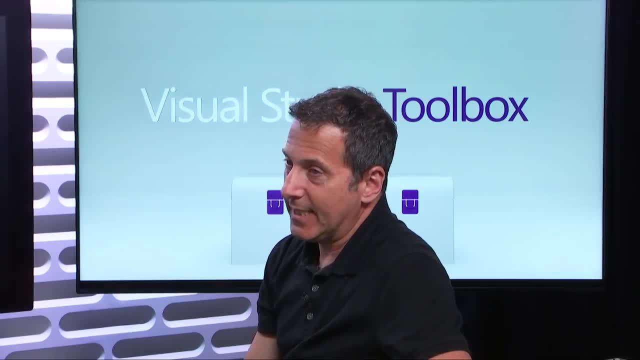 you're almost talking about what type of door, and not so much The door pattern. is that there is a way to get from room to room that can be closed behind you? Yes, Right, That's the command, that's the pattern, that's the door pattern. 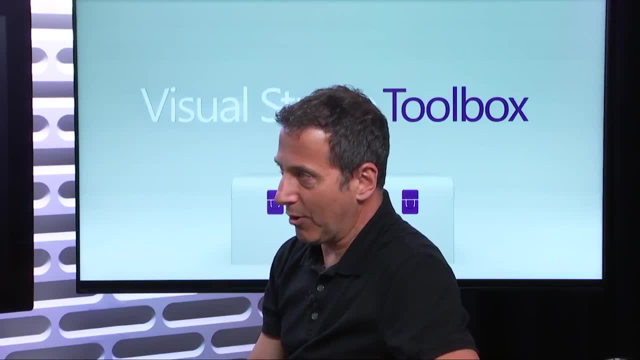 So we could say that the command pattern is: you encapsulate code, you call a method of something else. Yes, Now, on top of that, there's additional techniques and they have their benefits and we can just, you know, Yeah, Yeah. 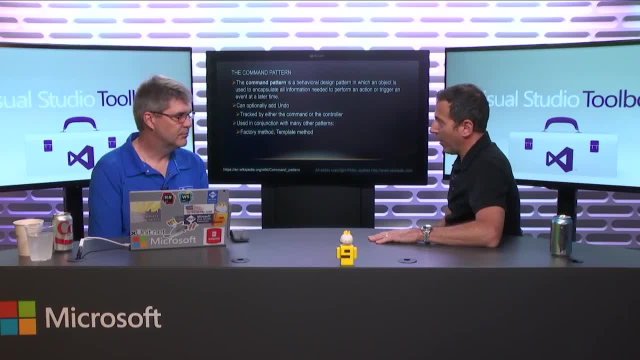 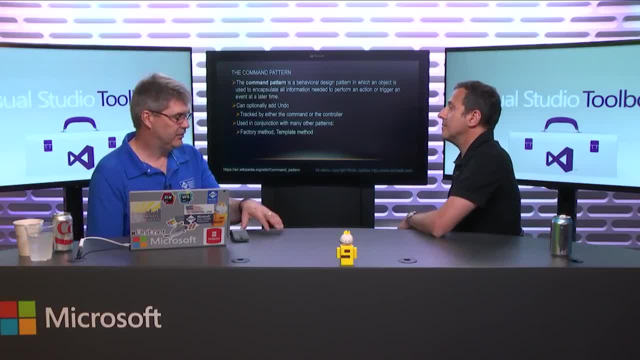 Right, Separation of concerns and single responsibility- Yep, The button. it's only job is to phone home Right. Or phone that weather service- Yep, Don't even know what weather service It says. get me information And in the weather service and we can talk about the factory pack. 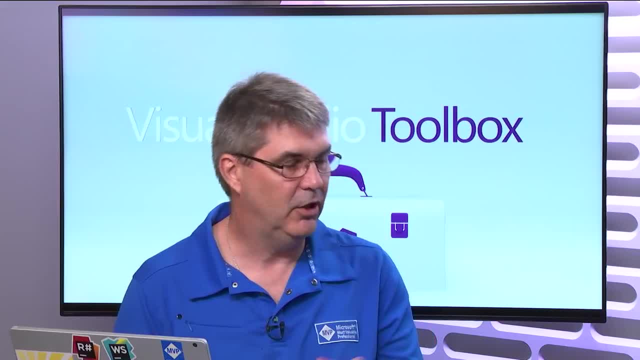 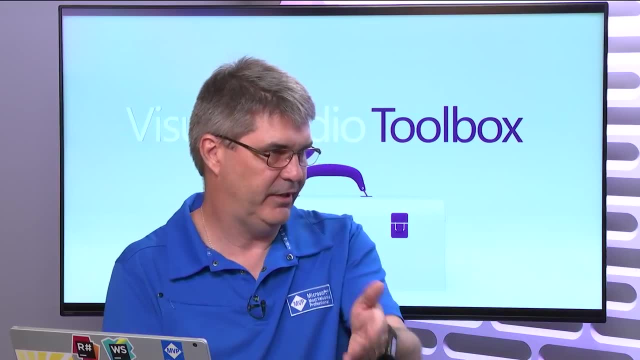 or we will talk about the factory pack in a later episode- can say: oh, which weather service would you like? Right, Right, And let me help you get the right weather service. so then you can make that call. So MVVM, MVC essentially automatically put you into this. 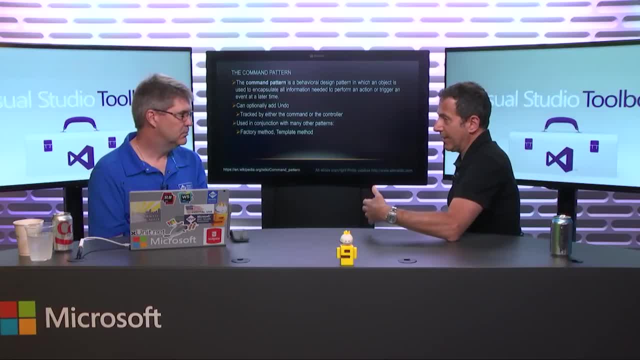 because in the code behind, all you're doing is calling a method of the view model, Right, Right, Well, and if you're doing WPF or XAML, That's the command pattern, right there. Absolutely The way buttons work in WPF or XAML. 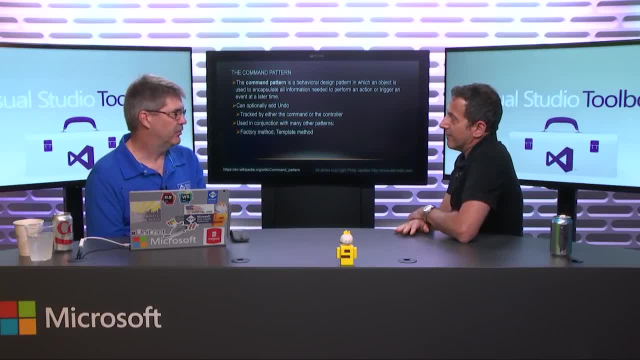 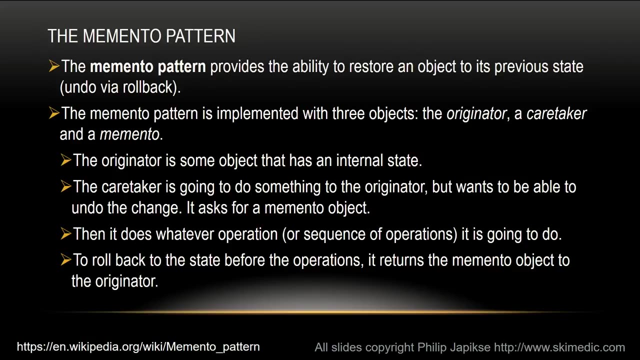 it is absolutely the command pattern, Right? Yep, Cool, All right, Let's go on the memento. The memento pattern actually does stand on its own, but it works really well with the command pattern as well, And what really matters is just that first sentence. 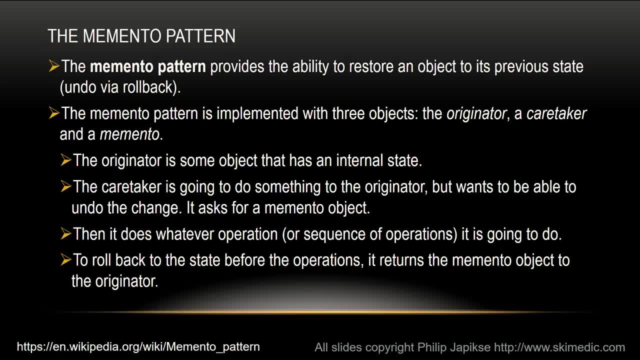 Again, lots of words on here that your viewers can read at their leisure, or they can hit pause on their computer and read it and not have to try and read it while I speak. But the memento pattern, I'm sorry, XAML, it is absolutely the command pattern. 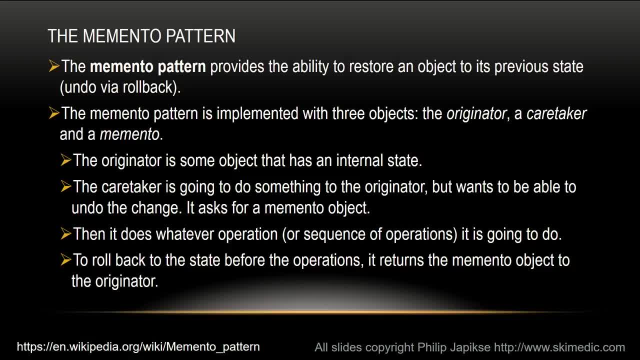 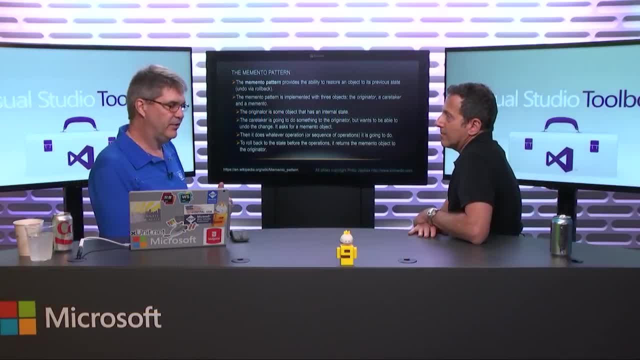 Right, Yep, Cool, All right, Let's go on the memento. The command pattern, easy for me to say, provides the ability to restore an object to its previous state, So it's an undo via rollback. Okay, Now how this is different than the undo we just talked about. 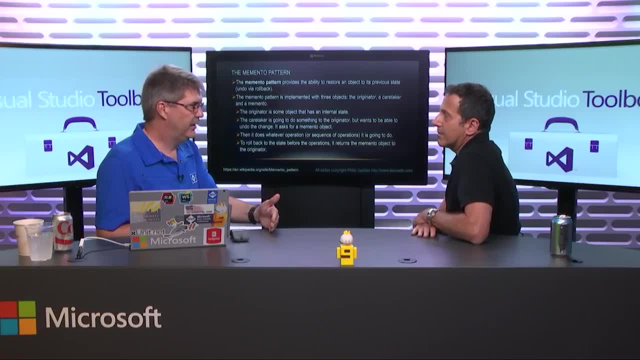 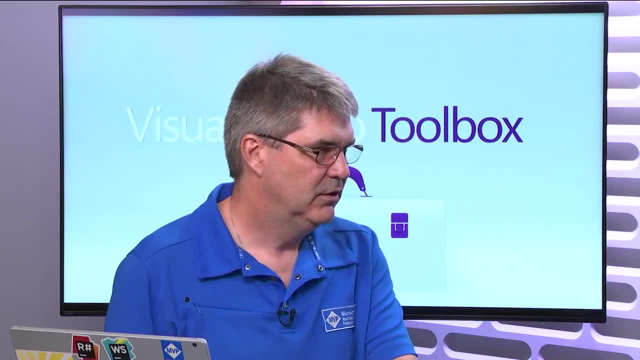 I was popping items onto a stack Right And then to do undo, I was basically taking them off or pushing them on the stack and then popping them off and then changing the state that way. Yep, This is actually saying what was the state of this? 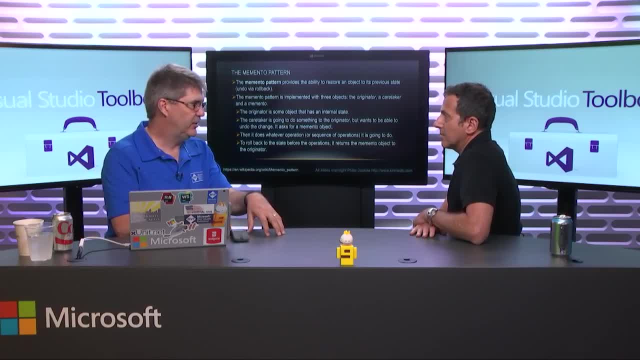 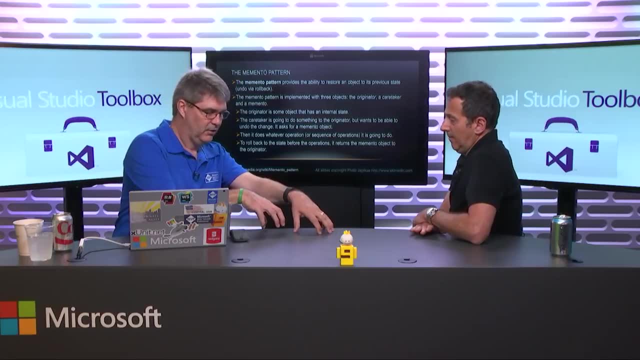 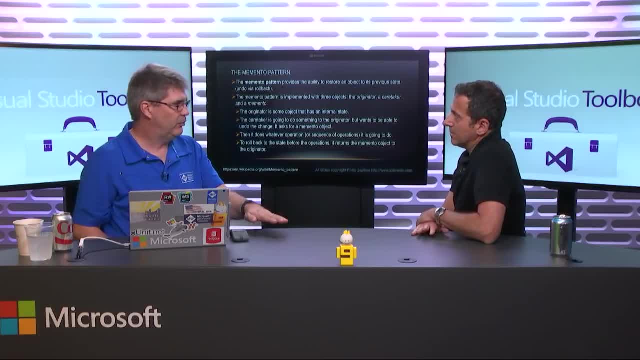 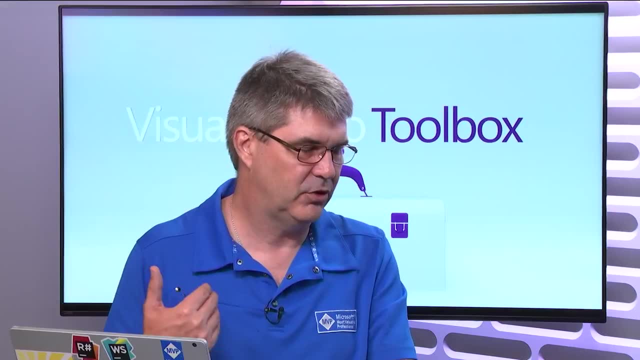 for example, how entity framework does it? So, entity framework, when you are tracking an object, you have the original values and the current values, And then of course you can make an additional calling at the database values. but that's kind of a different pattern. 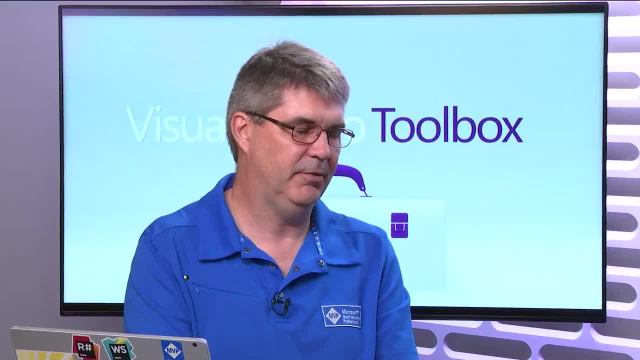 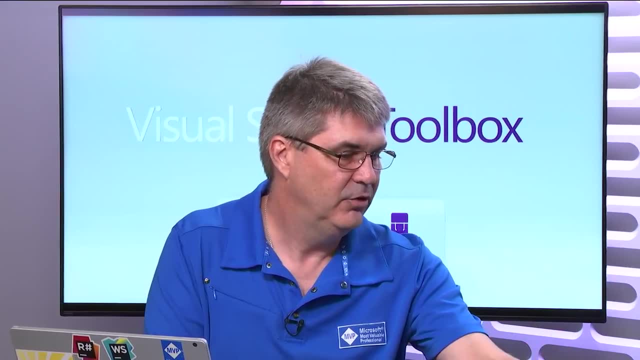 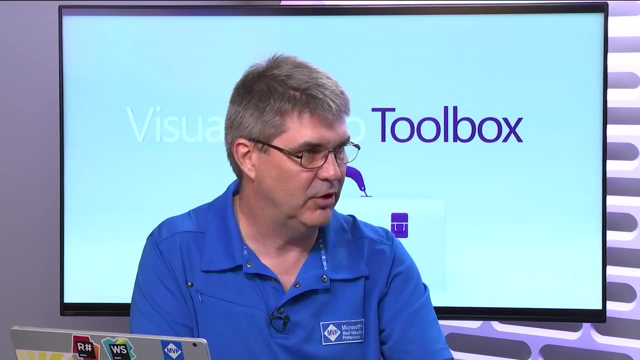 So I can undo, but the way EF has implemented it, which is perfect for that business case, undo says get rid of everything. roll me back to the initial state. So it's kind of the memento in that standpoint, but it's not storing all these states along the way. 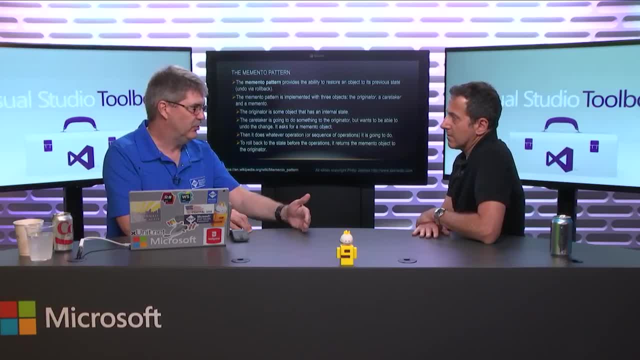 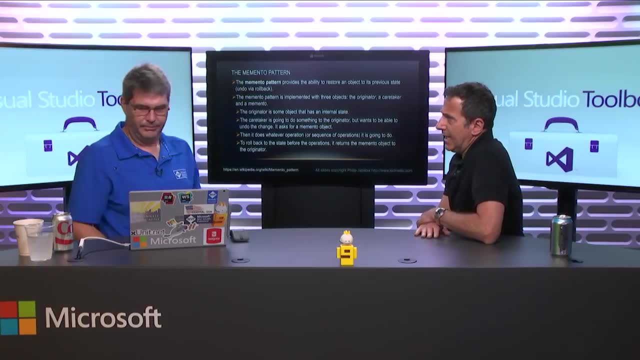 There's a good reason for that. If it's storing all these states along the way. guess what I've just used up on your computer: Huge amount of memory, Huge amount of memory Disk space, and it's also not. it's unintuitive, right. 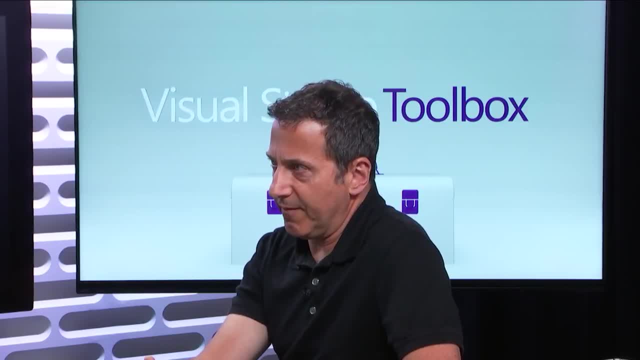 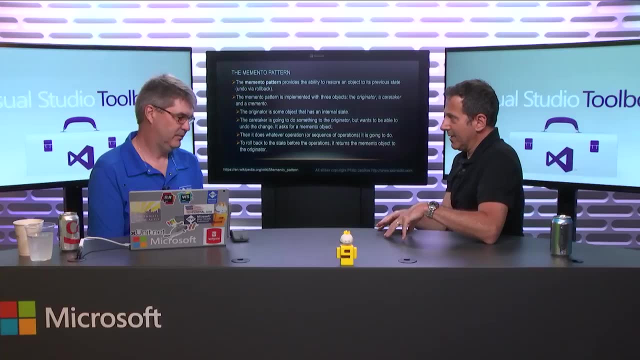 Correct. I mean I haven't changed the data until I save back to the database, right? If I'm in between, I'm undoing typing. I've done Yes, I haven't done the database. there's nothing to undo. 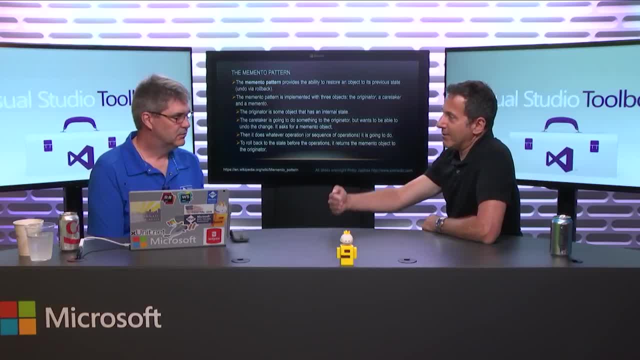 Right. So it totally makes sense that you would roll back to a save point. It's like checking in code, right. Yeah, Roll back a commit. I don't roll back the code I typed. You can't roll back the code you've typed. 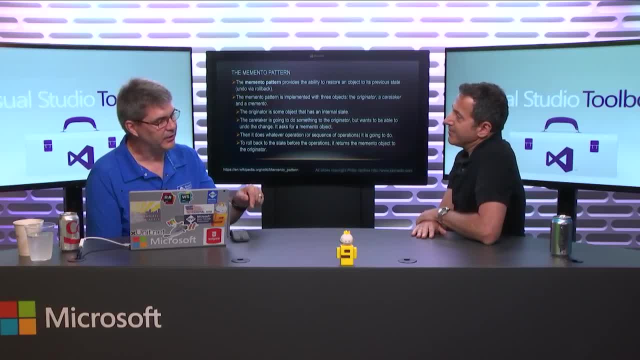 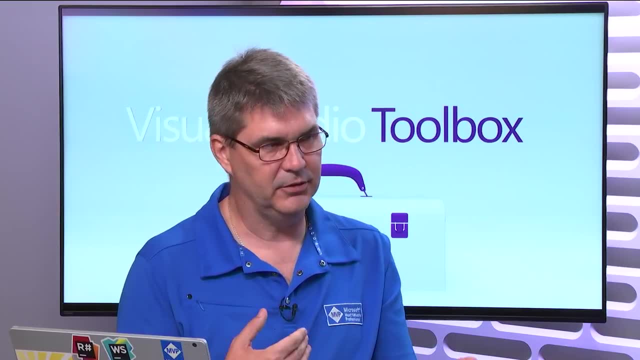 you can only roll back commits, Right. Well, but I can actually undo a particular change as part of a commit, right. Yeah, true, And so there's kind of that blend right, I can get back to a previous state. 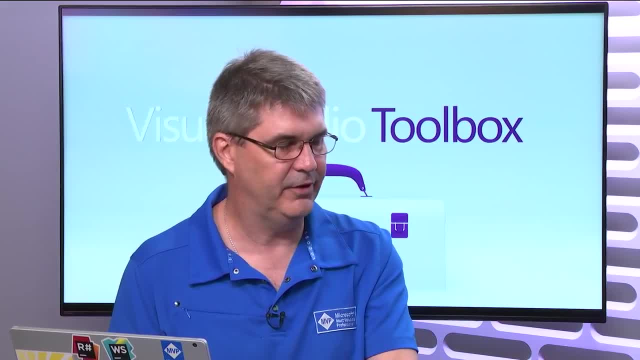 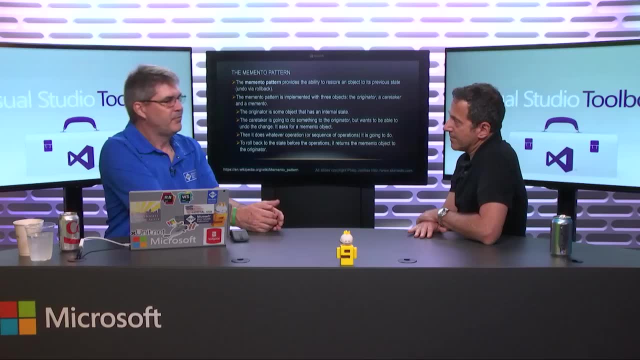 Right, But not the 27 things that I typed undo those, but keep the first 43 that I typed Right Or something crazy like that, right, Right. So it's standard. It stands on its own. the memento does. 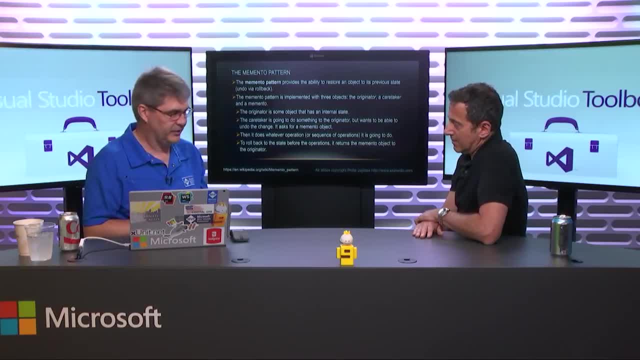 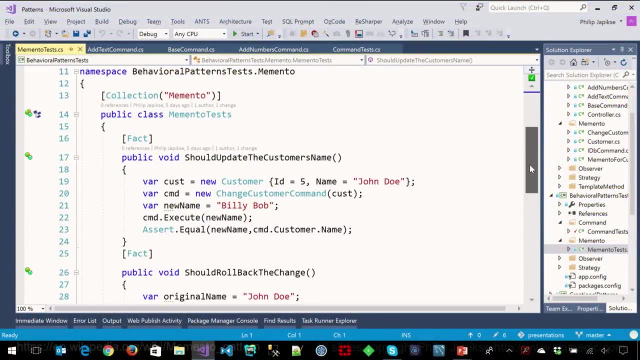 and you have to really think about what's the business case for using it, Right? So if we look at this- and this is why I like talking about this with the command pattern, because it's a great way to demonstrate it- You can usually tell the command pattern because 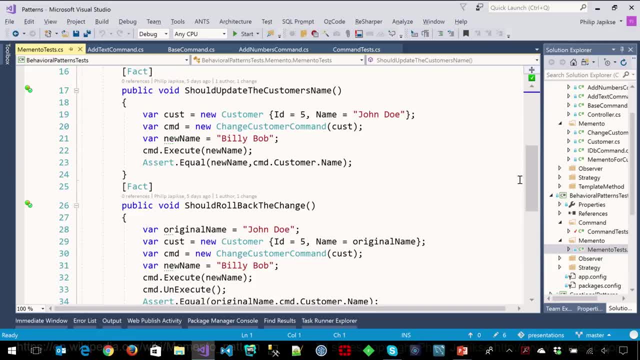 something is going to have the word command at the end of the name. Of course naming is hard. So I have a new customer object, very simple customer, two properties, and I have this change customer command and execute just changes the name. 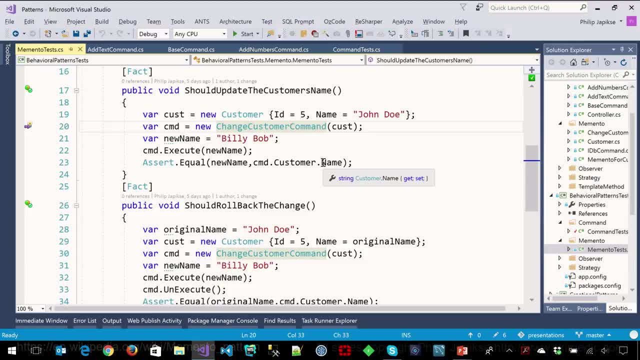 Again, very, very simple example probably wouldn't even need a memento or a command to just change the name. I could just change the name, but I wanted to demonstrate the pattern. So then I assert that the name was changed. Yes. 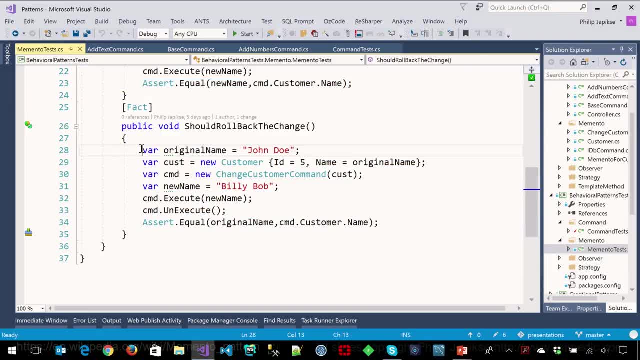 But here I want to do a rollback. So here I have: the original name is John Doe, On line 29,. I create a new customer On line 30, I then change it or create the new. change customer command. So those first four lines. 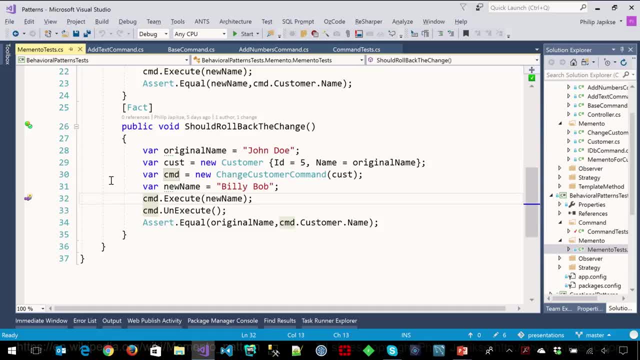 five lines are essentially the same. Only difference is that I put the original name into a variable because I need it in my test. I then call execute, name becomes Billy Bob, but then I call unexecute and I want that customer to be exactly the same as. 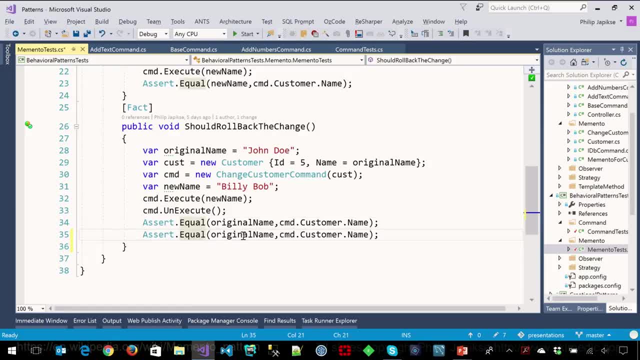 as it was Okay. So I can add an additional assert right here where I can say commandcustomerid is five to show that I'm getting back that complete state. Sure, This is where the memento shines, If I had 30 properties on this customer object. 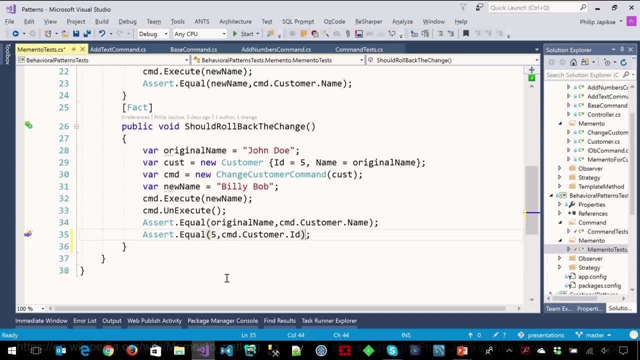 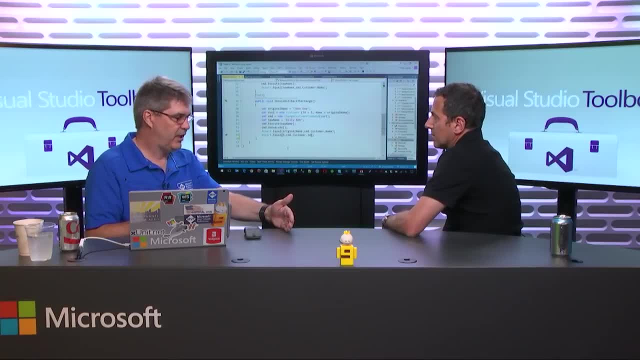 which one could argue that's too big, but it's either here or there and I had to return to some specific state. does that mean I have to track for every single property on that object? to change history and the change history in relation to other changes? 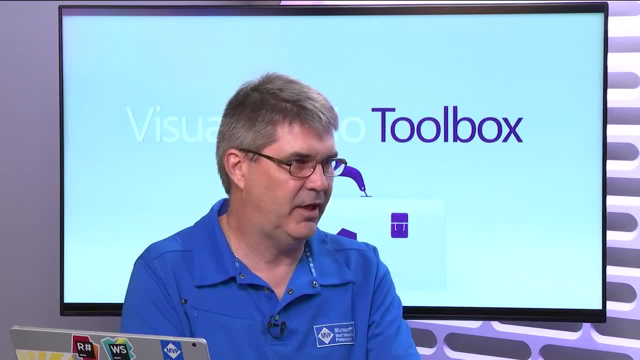 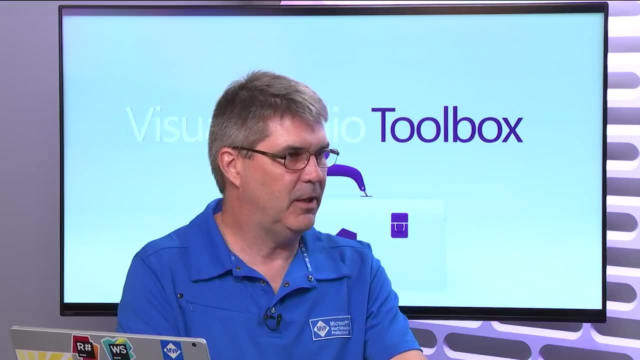 Well, I hope not Right. So I've changed the name seven times, I've changed the ID twice, which is evil. you should never change ID. but that's again another story, And now I have to sync it up. 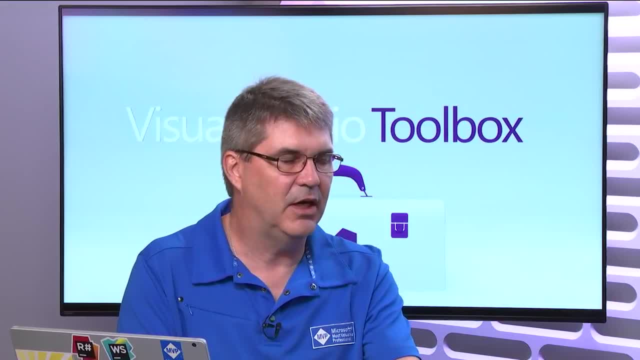 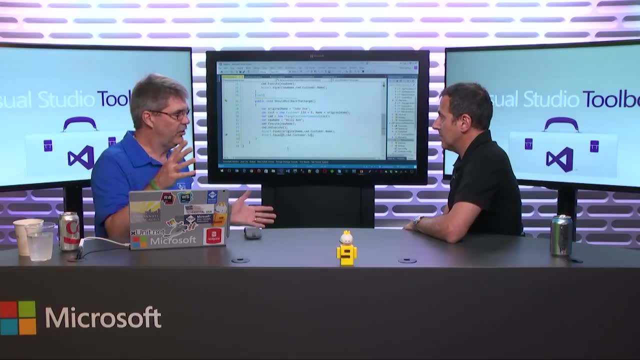 to whatever it was at this given point in time. Well, that's a lot of tracking and a lot of wasted effort, Whereas with the memento I can say: give me the state of the entire object at this point, this point in time, or back so many changes. 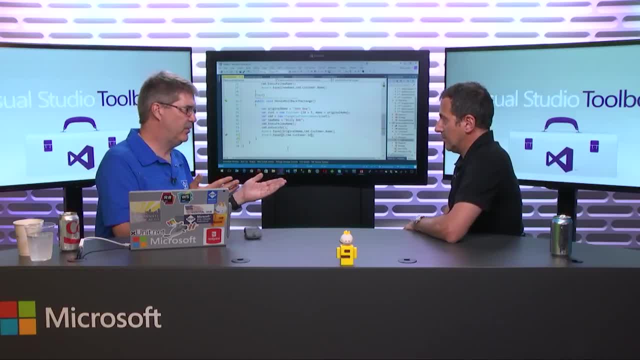 back seven changes. doesn't matter if six of them were the name and one of them was the address. Remember when we talked about the simple command pattern in the undo, we had a problem with that. Yeah Right, This fixes that. So let's look at how we do this. 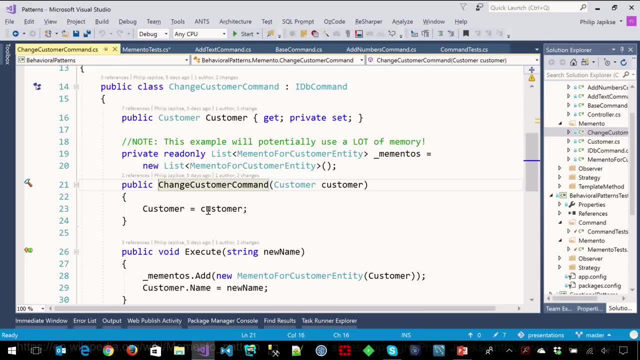 Again, a simple command. I don't need to go into there, But I have, instead of a list of entries, I have these memento for customer entity classes And that's what I'm tracking, as opposed to specific changes. So when I change the customer, 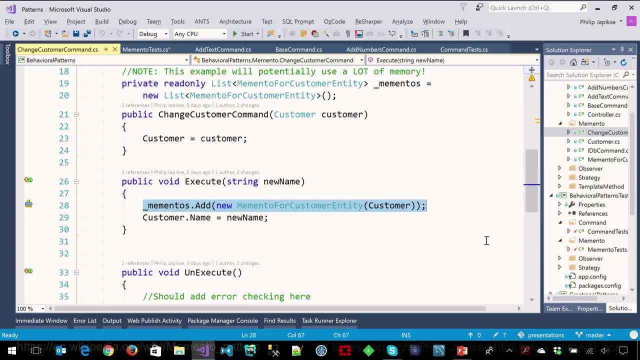 before I change it, I add the current state into a memento object. Okay, And then I make the change And you don't just add the customer, I don't just add the customer. We'll talk about it in just a minute. 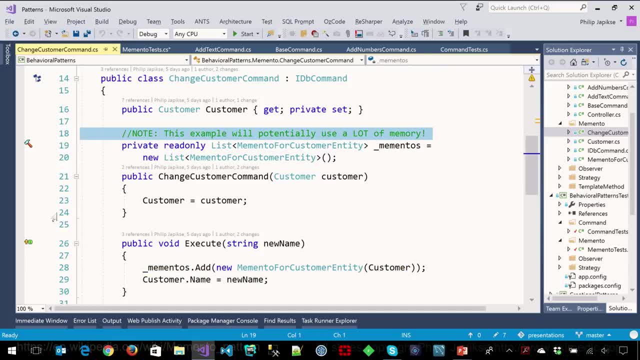 But I will point out that this example can use up a lot of memory. Again, I just want to show an example of how this works. One specific implementation: You can write it to the disk. if you are concerned about that, Yeah, There's a number of ways to do that. 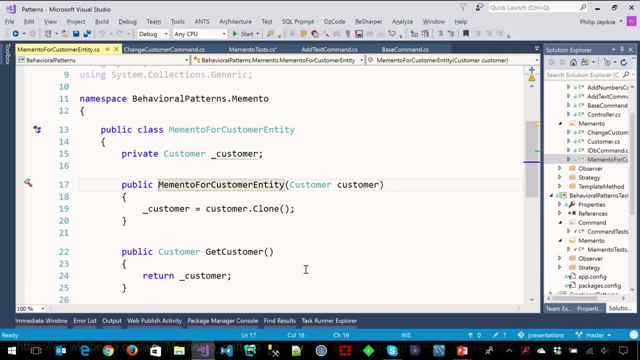 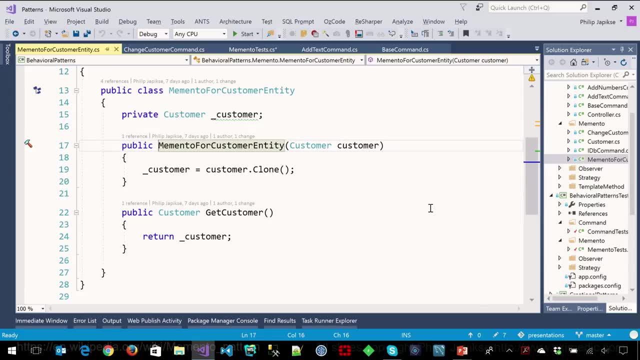 So let's look at what a memento is. So memento is just a way of maintaining state for an object at a point in time. You had said a great point and you're almost like a big man leading me right into what I was going to say. 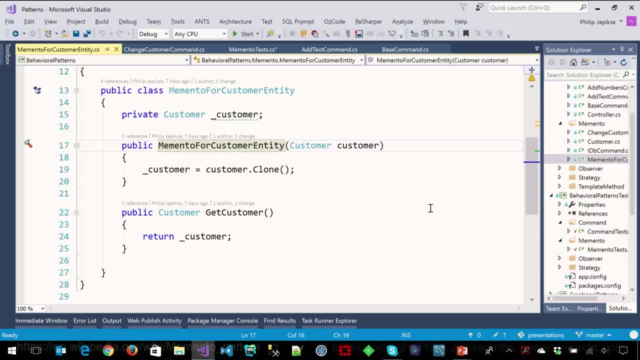 For you younger viewers. never mind If I just saved a customer. the customer is just a pointer to a variable on the heap Right. So if I'm saving these customer variables, then they will get changed along with the customer. So I actually have to create a clone of. 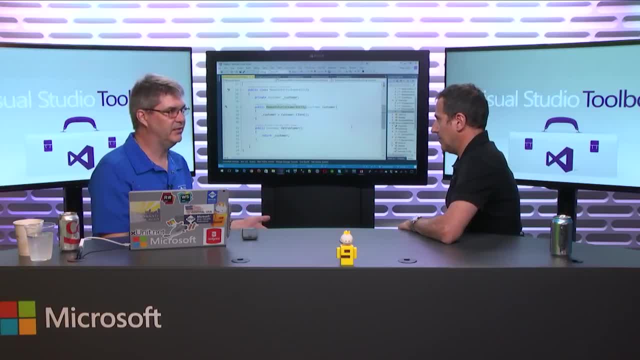 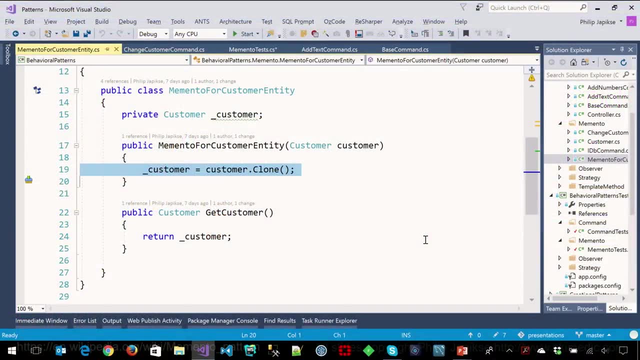 that customer and save that in order to get back to the state that I was in Right. So in this example, the customer knows how to make a clone of itself, as allNET objects do, Mm-hmm. So getCustomer just returns the customer.